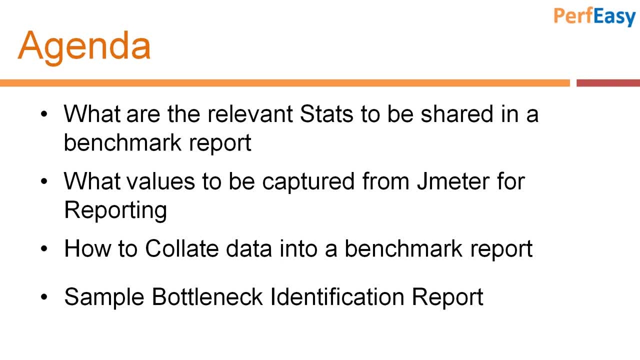 Result file to a CSV or an Excel sheet. Then we are going to like generate some charts, like observe some data and we are how we are going to present it in a benchmark report, or I would say a benchmark report deck. And at the end of the session I am also going to share or show you a sample bottleneck identification reports, because in a benchmark report you will not find the back end. 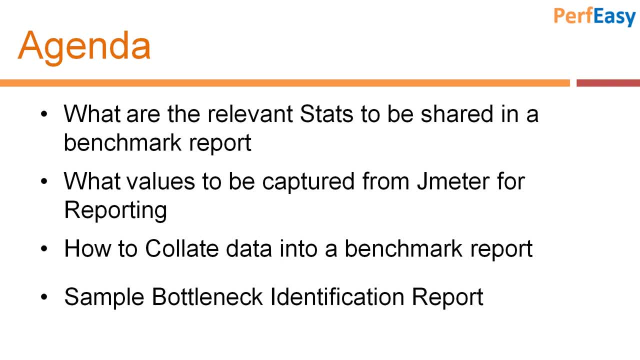 Data. when I say back end data, like in benchmarking, we only see which pages are slow or which requests are slow. But in case of a bottleneck identification activity, what we do is we also pinpoint the reason for the slowness. So in the code code, if there is any class or a method that is taking more time to execute or causing a memory leak, we share that. in a database, there can be a query or a missing index. 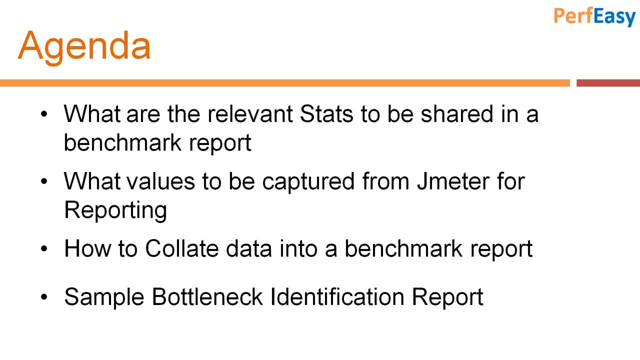 Or some memory issue or some deadlock issue that we identify and pinpoint. So in bottleneck identification report we have all these pinpoint issues are also shared and some observations and recommendations are also shared. So I will- I'm also going to share you a sample bottleneck identification report at the end of the session. 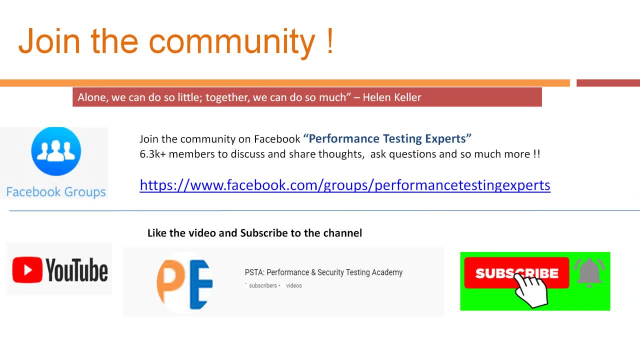 Before we move on, I would also like to share a sample bottleneck identification report. Before we move on, I would also like to share some information. like, we have a performance testing experts- This is the name of the Facebook group, or a community that we have on a Facebook, and we are like. more than 6300 members are there and we are sharing our information, the job post, as well as we ask our questions wherever we get stuck, and a lot of exciting things are happening, So do join in here and do not forget to subscribe to the channel. 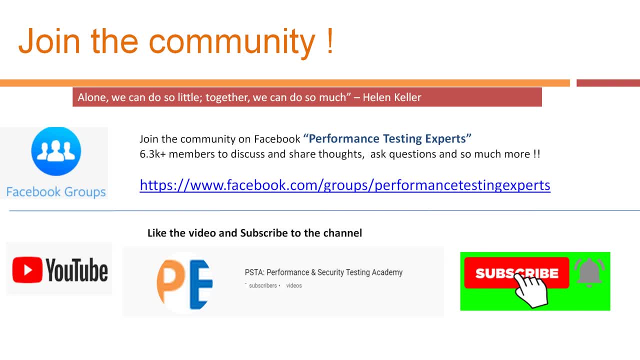 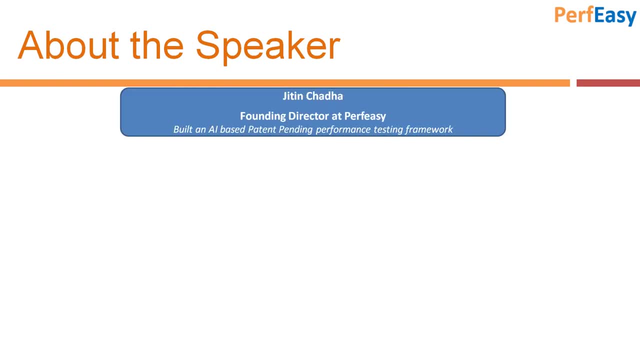 Like this video and share with people whom you think can get benefited from this. A quick introduction about myself. I am Jitin Chadha. I am founding director at PerfEasy Enterprises Private Limited, which is a Noida based QA testing organization, So we provide software testing services, including performance, security, automation, VAPT. 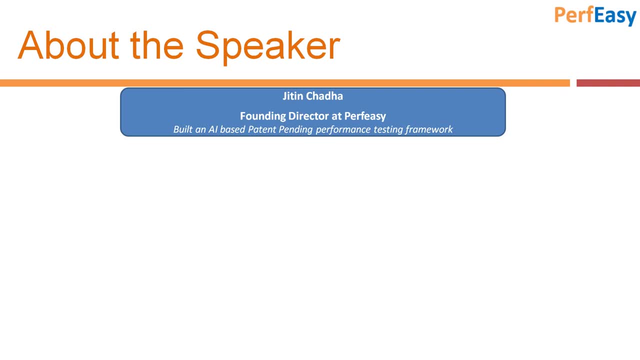 Usability manual. so if anyone has any requirement for testing activity, we definitely would have the solution for you. For more information about me, I have around 15 years of experience in performance and security testing. I have completed around 150 plus assignments. I have worked across the technologies like investment banking, insurance. 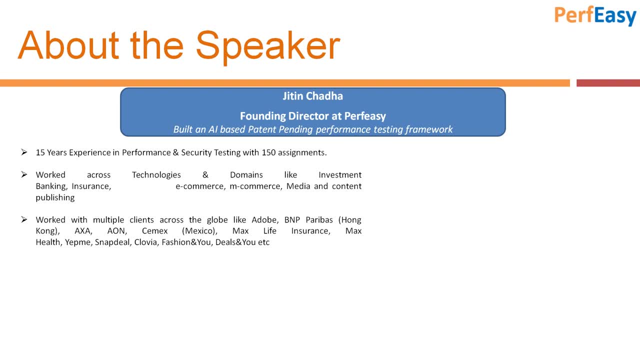 e-commerce, m-commerce, dotnet based applications, java based applications, php based applications, nowadays the nodejs socket based. so a lot of things i got chance to work on. i have also worked with clients across the globe like adobe, bnp, paribas, exa, aeon, samex, maxlife insurance, clovia. 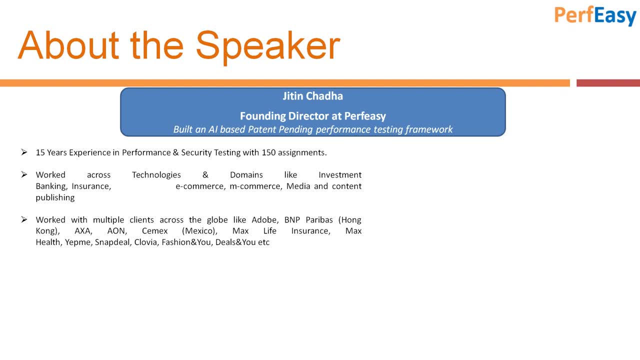 some e-commerce clients like yepme fashion and you, clovia, snapdeal. some insurance clients like maxlife insurance, aviva life insurance, max healthcare- i have also worked so- and many more clients. some certification that i have are: hp loadrunner, ais, ibm certified solution designer. 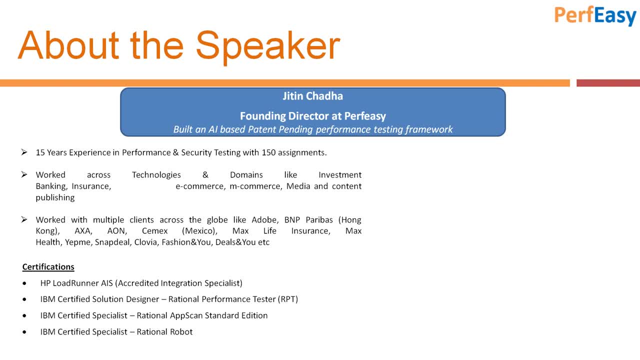 rpt. ibm certified specialist for rational app scan, which is a security testing tool. ibm certified specialist for rational app scan for rational robo, which is mostly an automation tool. i am not sure if it is still being used anywhere, so i did this quite a while back. if anyone of you feels that i can be of any help. 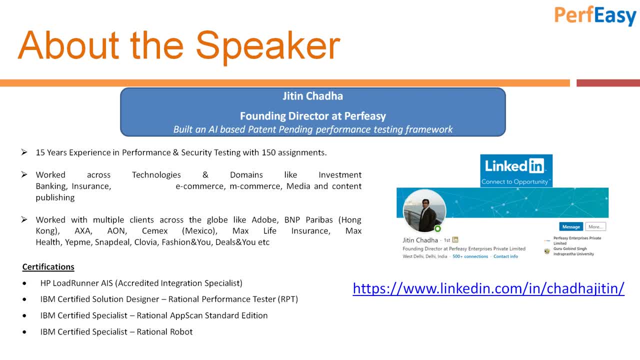 to you. please do not hesitate, connect with me on linkedin or a facebook, anywhere, and i will try my best to help you out. now let's move on to the topic of the today. so first of all, i want to, first of all, i want to tell you that i am a professional software developer and i have 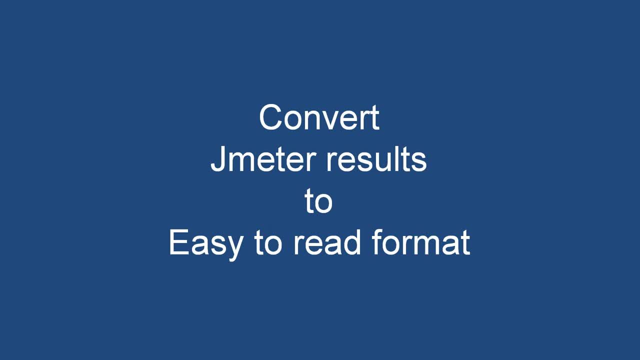 first of all, i want to tell you that i am a professional software developer and i have. first step we are going to talk about is how we convert the jmeter results to an easy to read format. so by default, jmeter produces a jtl file. the extension is dot jtl. so i am going to show. 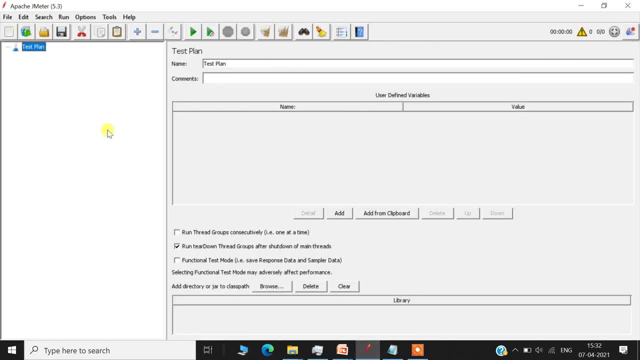 you practically how i am going to do so. this is the jmeter that i open. just click on the jmeter in the bin folder and this interface opens. so what i am going to do is i am going to add one thread group again, right click. i am going to add one listener. 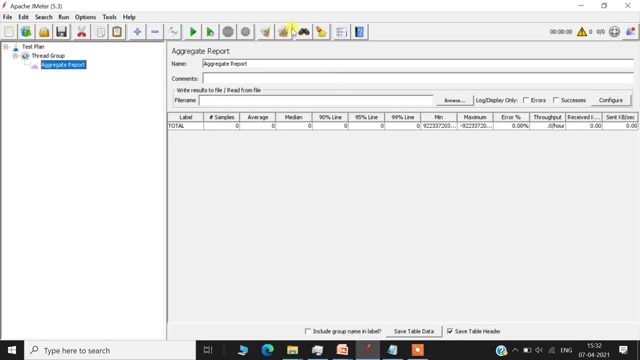 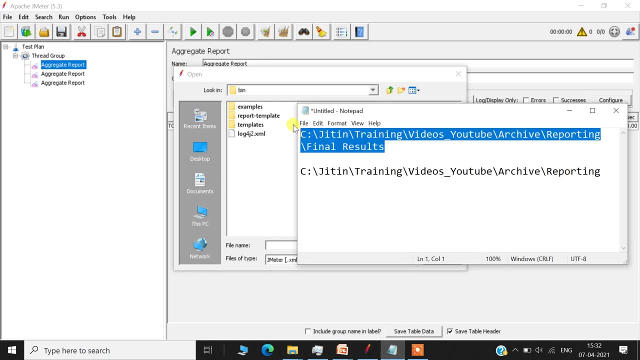 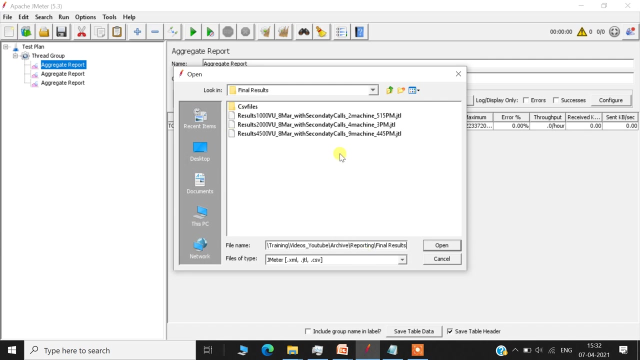 which is the aggregate report. i am going to create or add two more aggregate reports. so what i am going to do is i am going to browse and collect, or i would say fetch, the result files which i have already ran. so here i am assuming that you know how to run the load test and you have already. 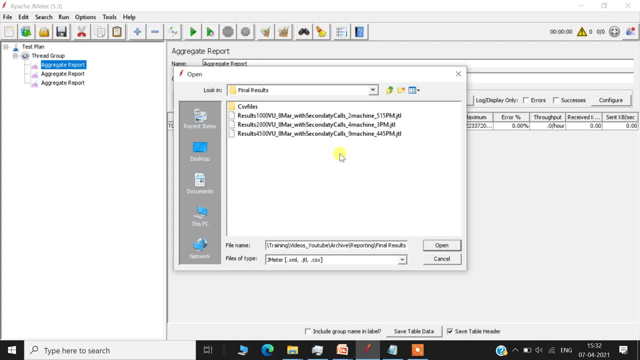 ran the test and you have the results. so here i have- i am going to use uh- three results. so make sure that you have at least three data points so that we can get a comparative analysis where, whenever we uh prepare a benchmark report. so this we i'm trying to set some context. so 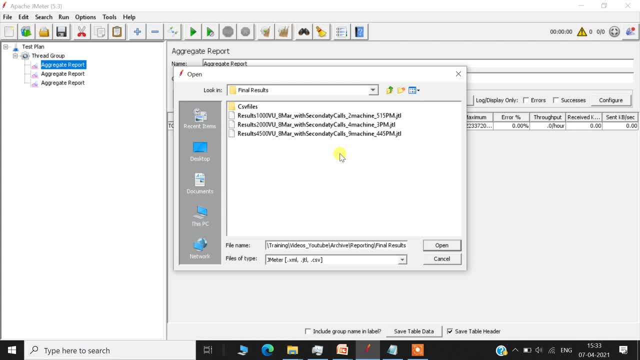 here we should always have at least three- and more than three- set data points so that we can get a comparative statistics. for example, here we have done a load test for 1000 users with two machines, if you see. uh, so this is like we ran this with a distributed load, so here we were able to generate around 400 to 500 user loads. 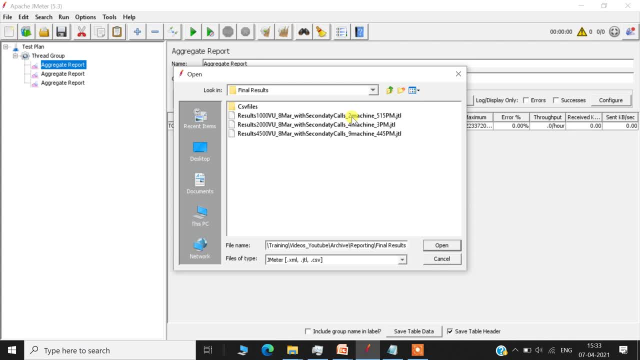 with one machine. so for 1000 users we needed, uh, two machines. for 2000 users we used four machines and for 4500 users we used nine load generator machines to generate that kind of a load. so we have now three set of statistics. so first i am going to select the first one thousand user load. 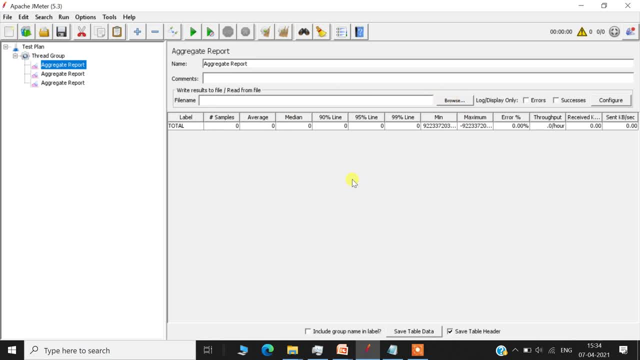 so what i did? i clicked on this browse, moved on to that folder where that jtl file was present and just select that file. so, uh, depending on the size of the result, the jmeter may take some time to load that data. so now, if you see, 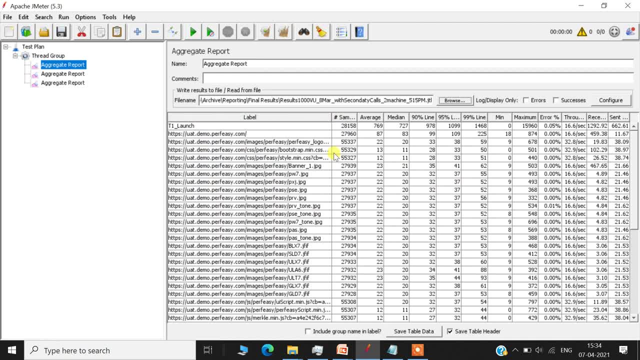 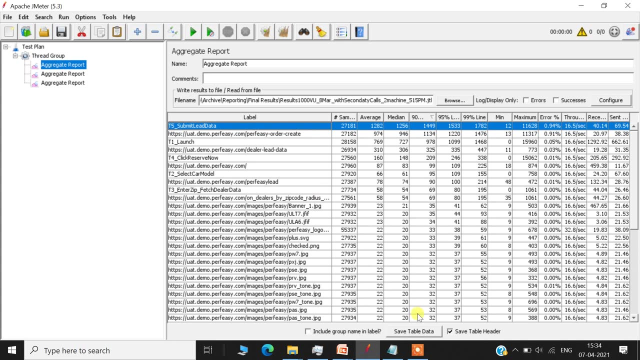 the complete data is loaded. so here, one thing that we need to uh, like before we should also do, is we should sort it based on the average time or the 90 percentile time, so that we can see which transaction is slowest. but here, what i am going to do is: i am going to so this is generated. i am 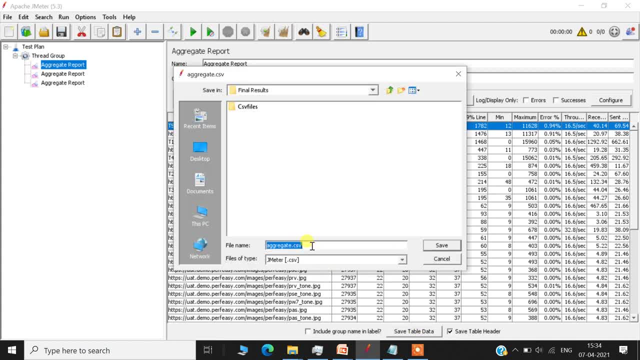 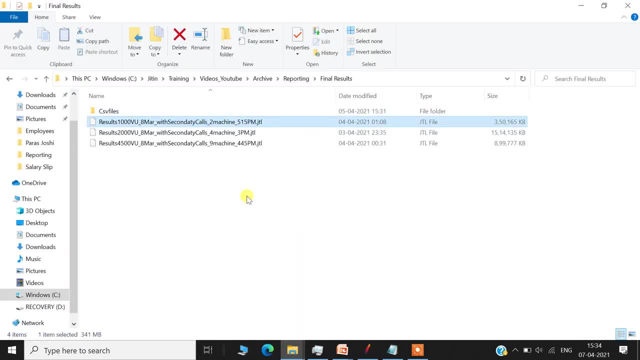 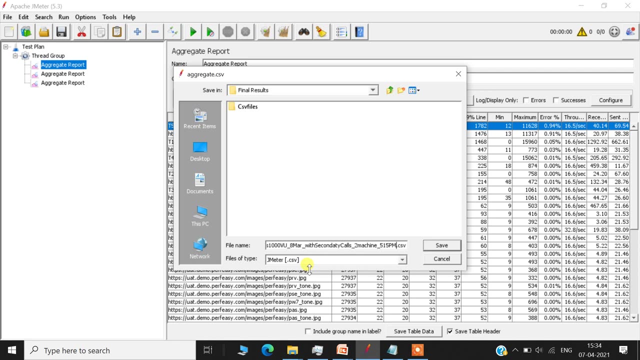 going to click on this: save table data. i am going to save this as a aggregate. uh, just what i am going to. i am also going to give it the name as the same so that there is no confusion. so i am going to aggregate underscore the same name, dot csv, so that i know this is the aggregate report. 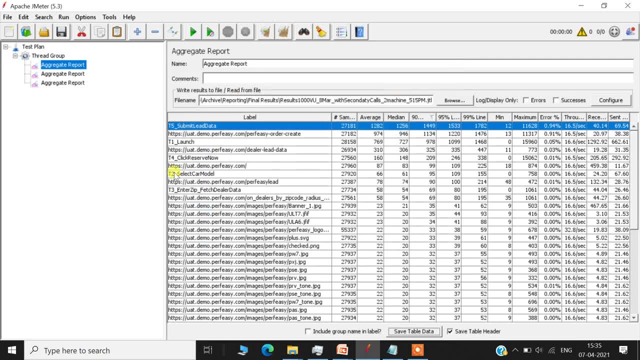 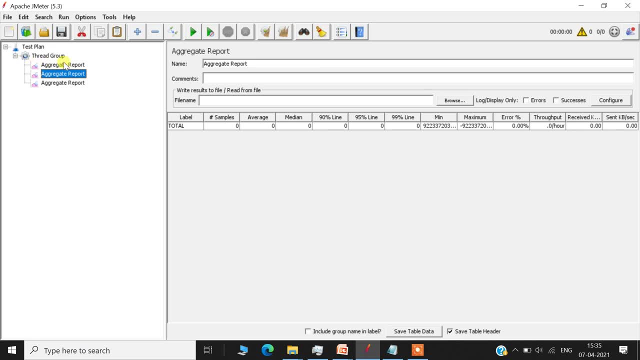 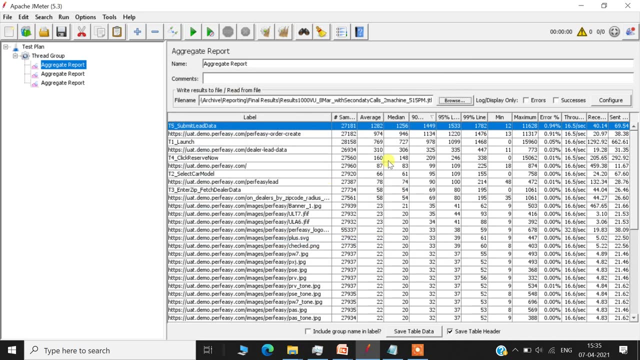 for 1000 users, so just click on save. now i am going to move to the second aggregate report, which is blank right now, so make sure you do not over write this. so, whatever, if i try to browse and add another result file here, what would happen? it would append the same data and the numbers would double up. so you 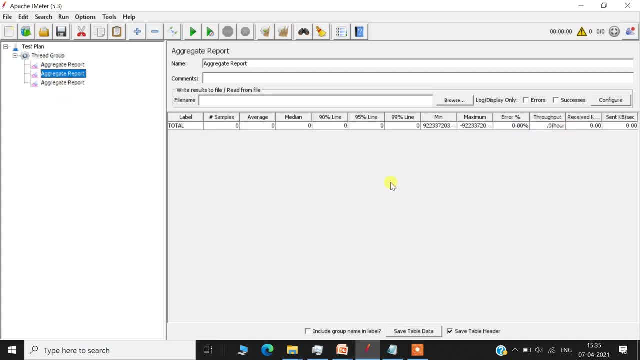 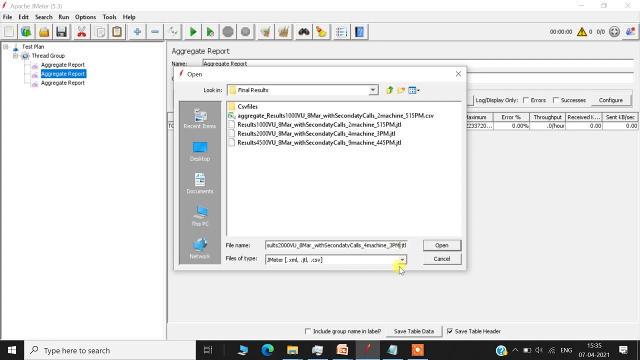 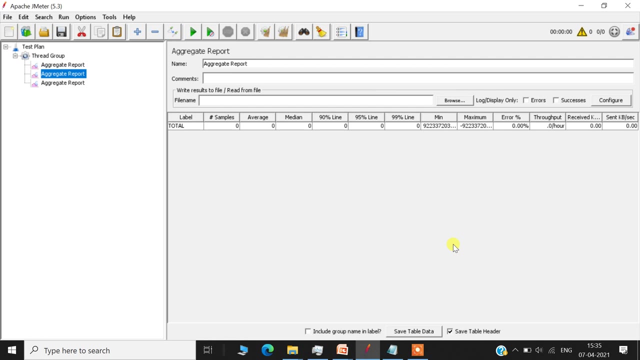 always use a clean aggregate report listener. go to browse. select the second one, that is a 2000 user file. i am going to copy the name only, so click on open. just wait for a few seconds to so that the jmeter is able to load the data into the jmeter, or this aggregate report listener. 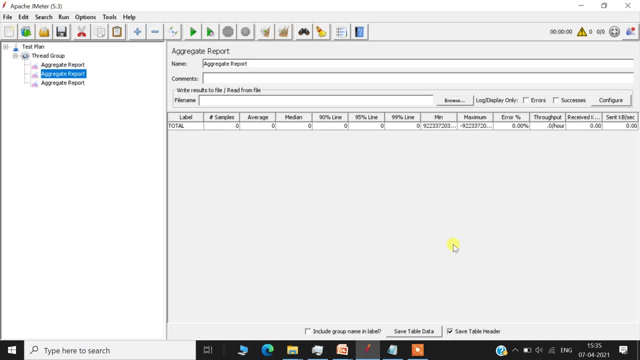 before we can create the csv file. so because the thousand user took lesser amount of time, because, uh, the the number of samples or the number of calls were lesser in 1000, while in 1000- 2000 user load, the number of calls would be. 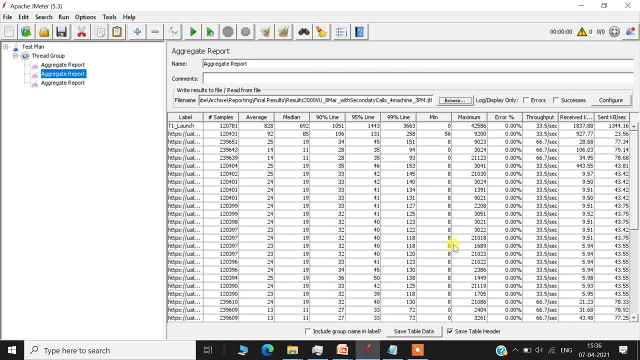 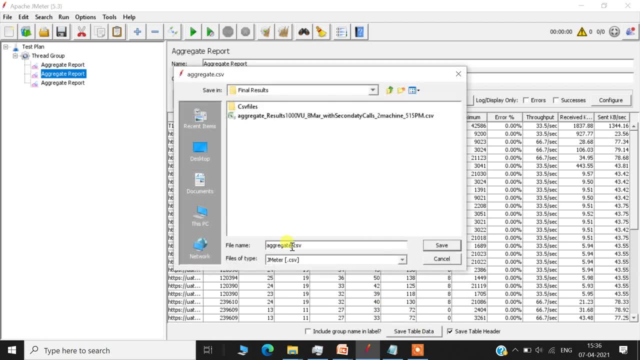 definitely be higher. so here it is taking a little more time to fetch the data or capture the data. so let me just click on again the same save table data. i am going to change the name: aggregate, underscore. the same name: dot 2000 view load. click on save. the file gets saved again. use clean or. 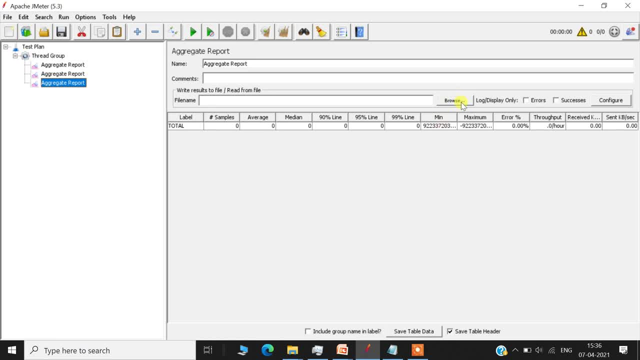 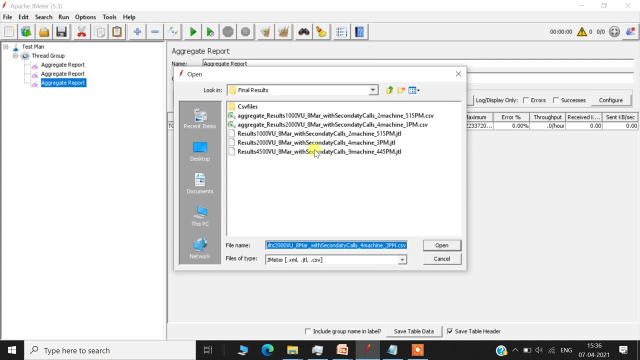 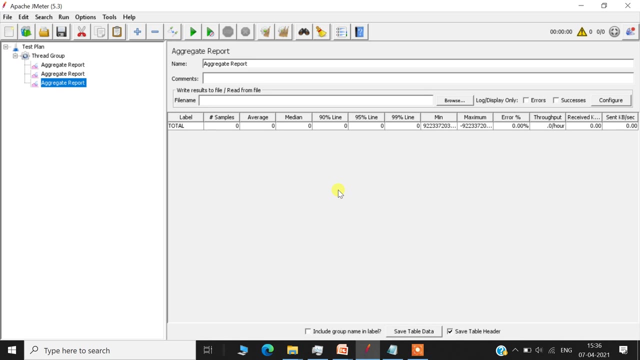 clear or without any previous data there. there should not be any data that is previously loaded in aggregate report. click on browse. select the third file. that is a 400 user load file. now it is going to load that file into this aggregate report listener, so we would need to. 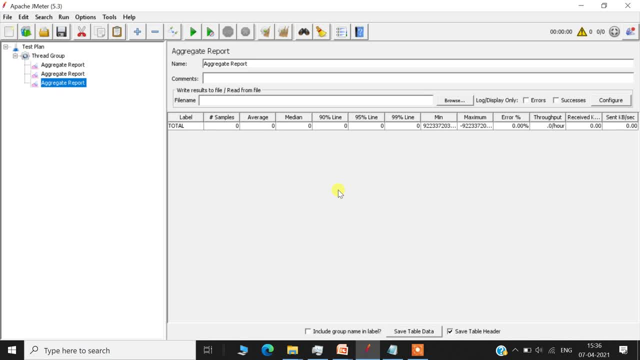 wait for a few more seconds so that the complete data get loaded by jmeter into this aggregate report file. so now, after this, once i save this data, i will have three csv files. my so, okay, so here, uh, so, uh, let's discuss about some things until the time this is getting loaded. 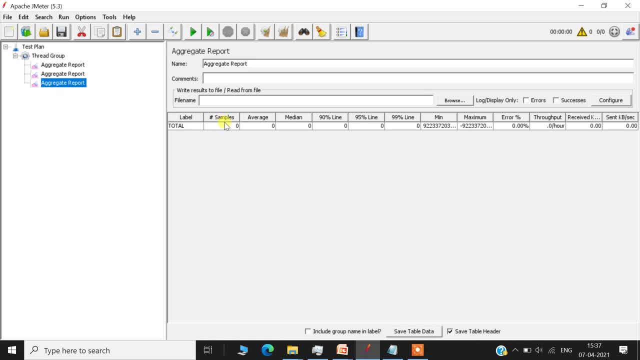 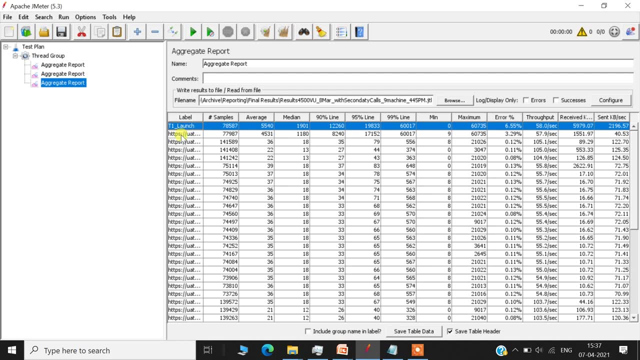 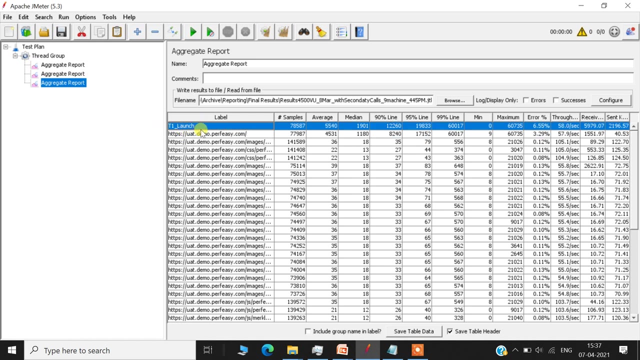 so here this hash samples is the number of calls that were made for a specific label. label is can be the transaction name or it can be the the number of calls that were made for a specific url or the request also. so this was: this is a transaction that is t1 underscore launch. 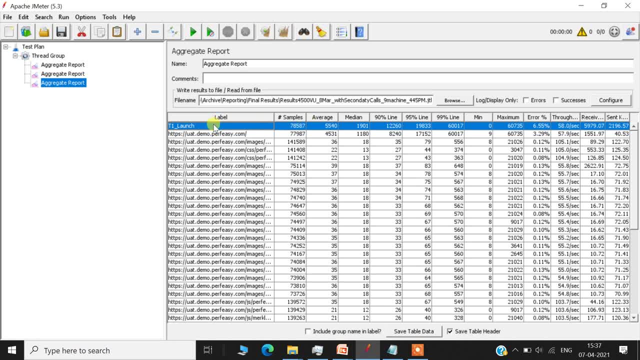 this is the number of samples, that is, number of calls that were made to the launch. this is the average response time in millisecond. millisecond is for seconds. we would need to divide them by 1000, so divide by thousand, so it means 5.5. second was the average response time for the. 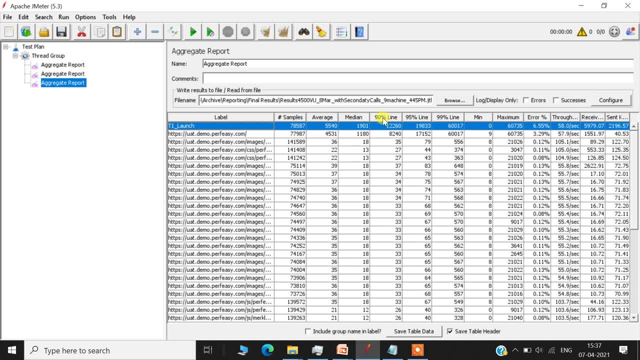 launch transaction. this is the median of the time. this is the 90 percent response time. this is 95. so, depending on what kind of or uh, what is the data that we are going to present, mostly we use 90 percentile line, but, uh, there are situations where we use 90 percent, 95 or average. 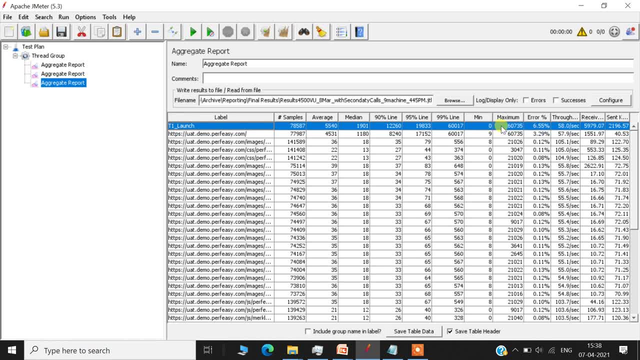 also. so this is the minimum and maximum response time that was uh uh captured. this is the error percentage. six point five, five percent failures were uh uh found in the launch transaction only. this is the throughput. this is the receive bytes per second. uh, let me just make it a little bigger so that we can see. 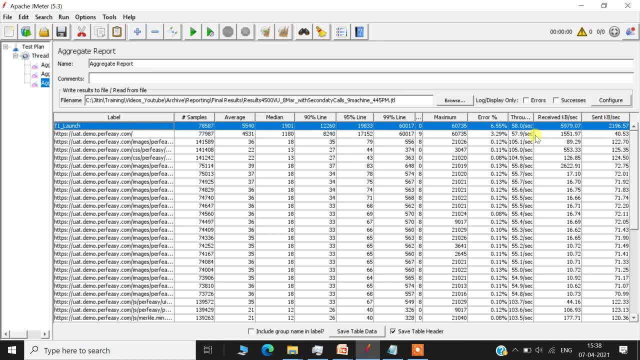 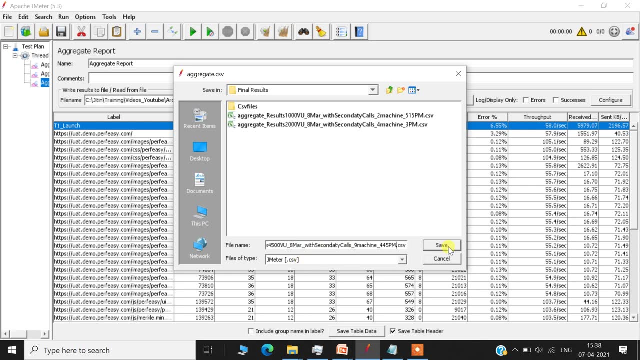 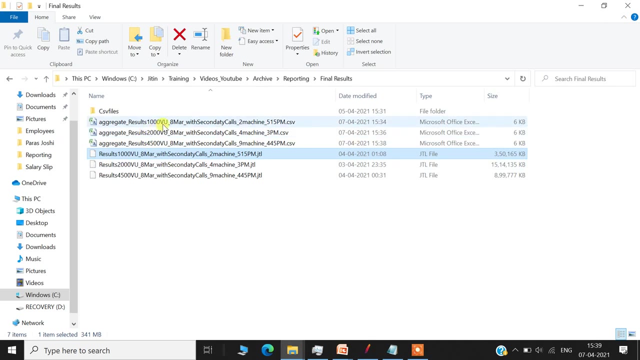 received kb per second here. sent kb per second, so let me save this data also. i am going to copy the name so that again the same thing: aggregate underscore. same file name: dot csv. click on save now. let me move to the folder. if you see, now we have three csv files. 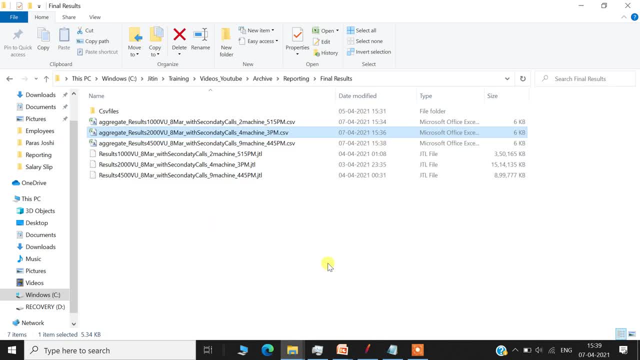 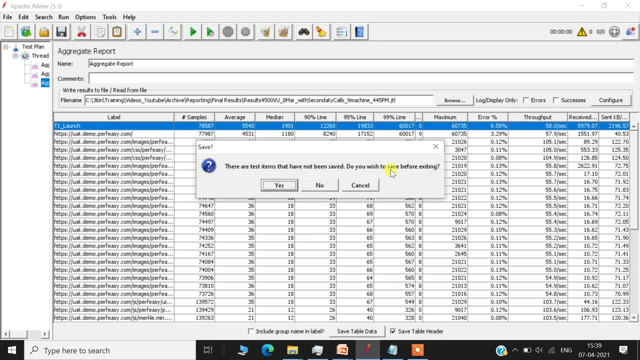 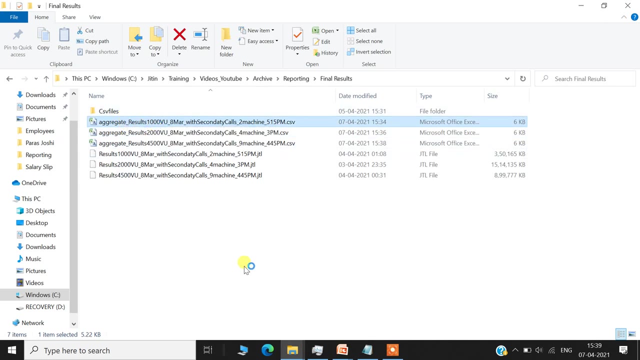 for 1000 user, 2000 users and 4500 user. let me just close jmeter so that the resource consumption on my machine is reduced a bit. so what i am going to do is i am going to open this 1000 vu file. 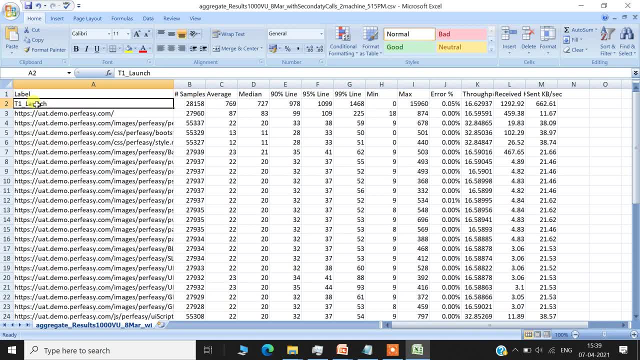 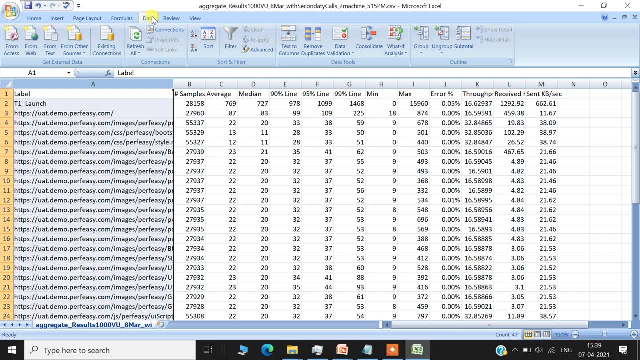 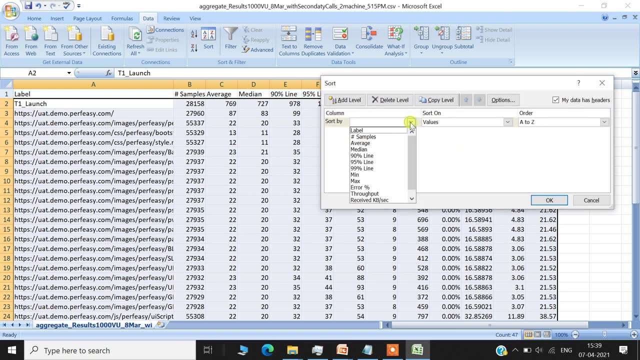 while we were preparing the script, we gave each transaction a number, if you see t1. so what i am going to do is: i am going to go to data sort, expand the selection sort by. i am going to do with label, because i already so, while in the 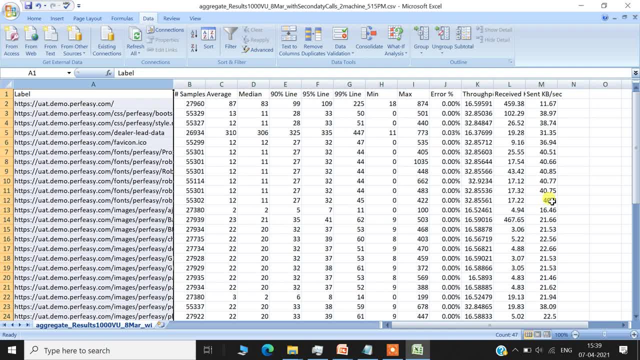 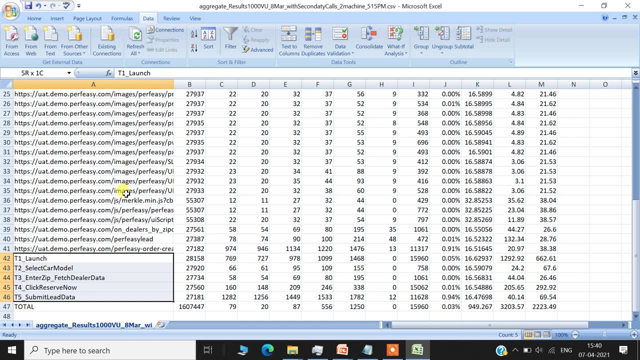 scripts only. we gave the names as t1, t2, t3 for all the transactions. let me go down at the end. so if we see t1 is launched, t2 is select core model, t3 is enter the zip code and fetch dealer data. fourth, or transaction four, is click reserve now and the transaction five is submit lead data. 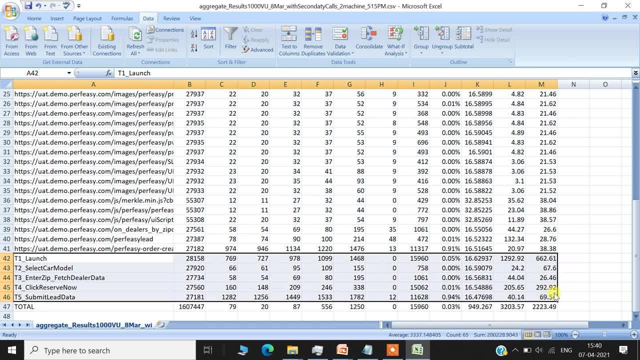 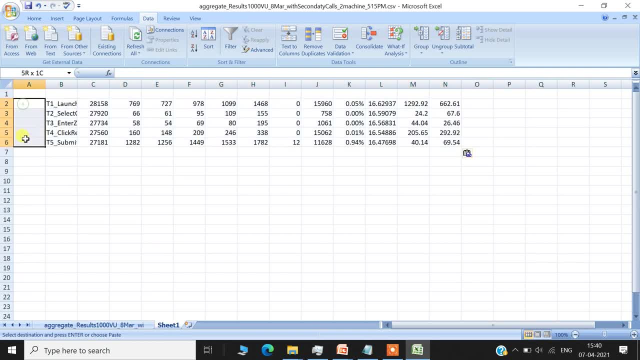 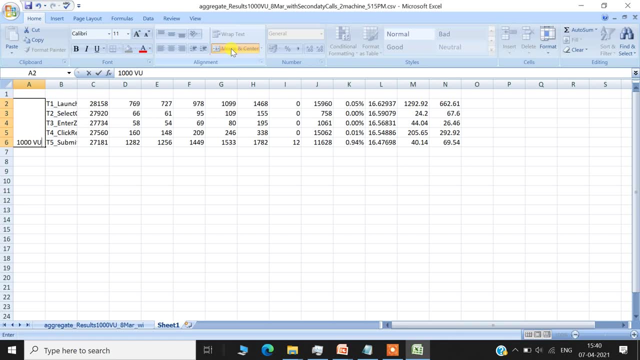 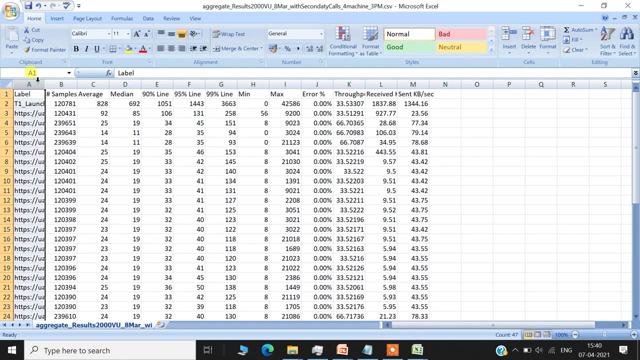 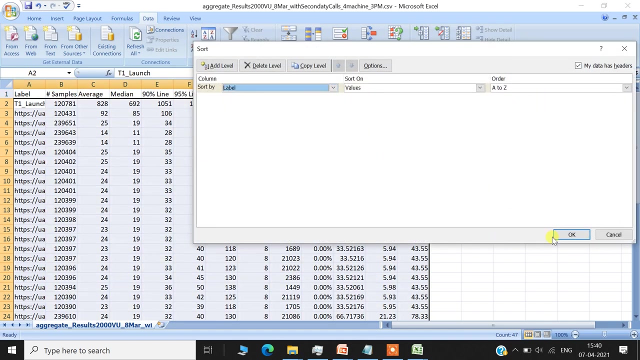 i am going to copy only this transaction data. let me copy this to another tab first. so this result is for 1000 vu. let me open the 2000 file result file. here also i am again going to do the same steps, sort using label a to z. so my labels are found at the end: t1, t2, t5. i am going to copy. 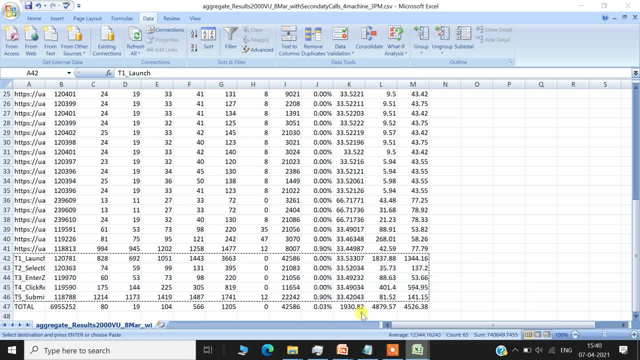 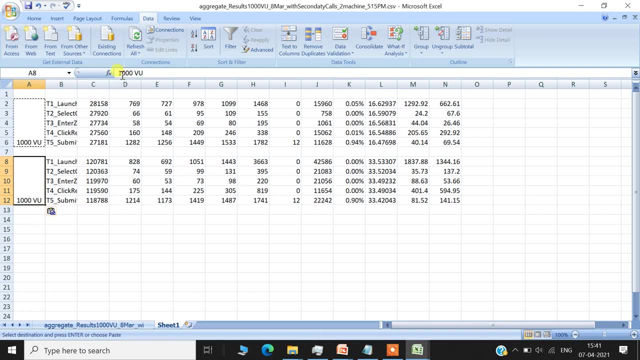 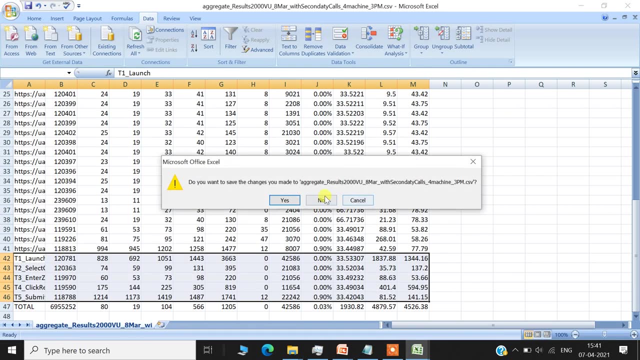 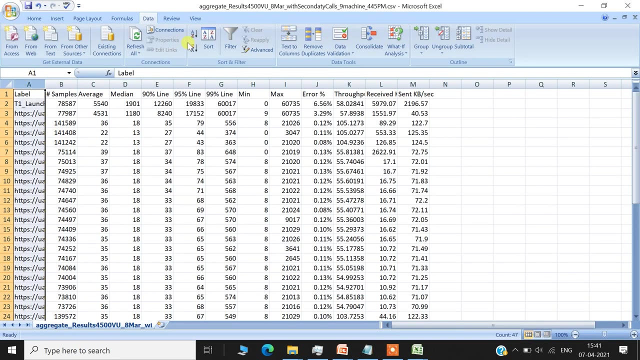 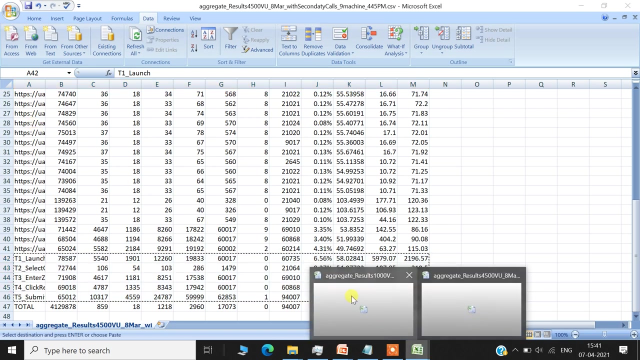 the complete data into the same place. in place of thousand i am going to make, change it to 2000, close that to a thousand view file, open that 4500 view file. again the same things, sort, sort by label. okay, go back back page down. so t1, t2, t5, all the five. i copy the data into this first file. 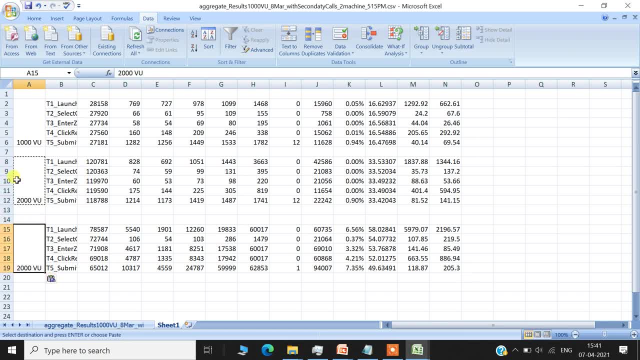 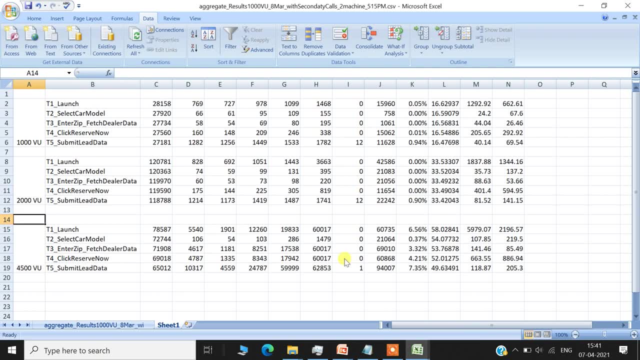 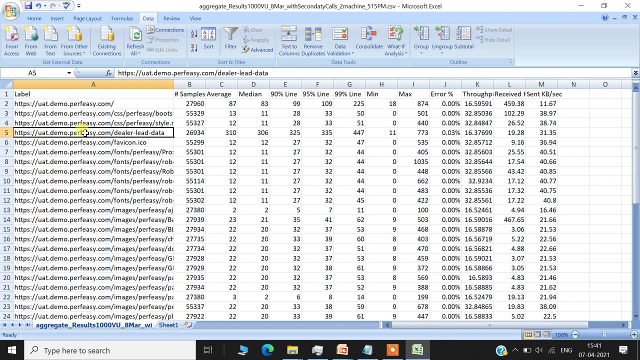 here, in place of 2000 i am going to mention as 4500. so now i have data with me. so when i say data, let me just close this file. first, let me go to the first sheet and copy this so that we do not get confused. 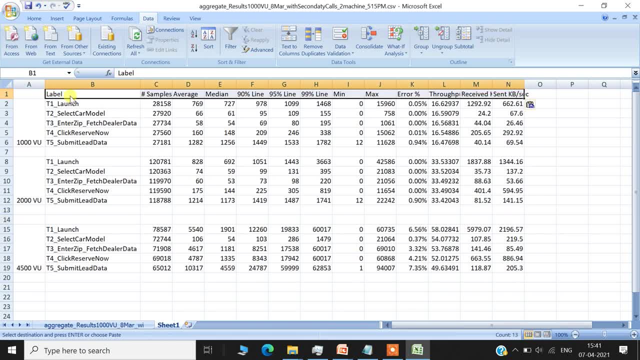 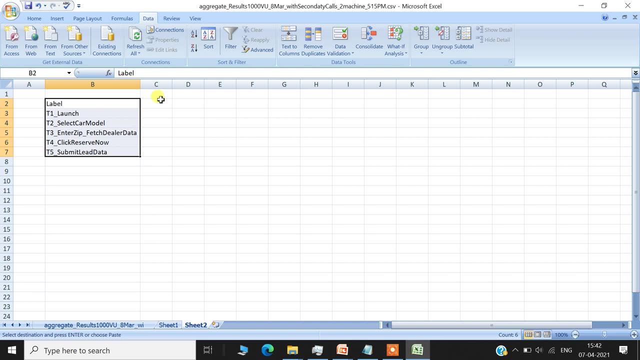 used with the columns. So first I am going to use the name. let me another sheet. I am going to copy the names of the labels. Second, I am going to like. first I am going to compare the response time statistics. So what is the response time? increase in the response time. 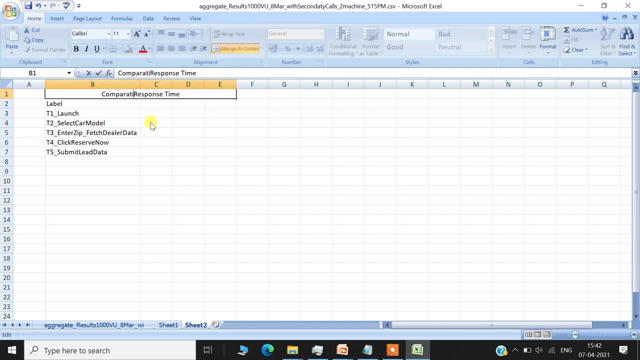 Or I would say comparative response time stats. So here after this, we should be able to see how much response time increased when we moved from 1000 users to 2000 users and to 4500 users. Was my application getting slow or the results were same. I am going. 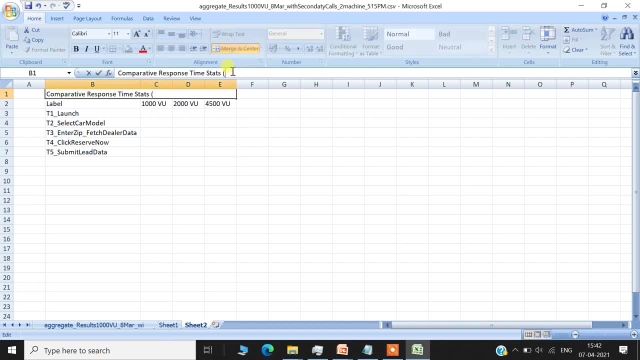 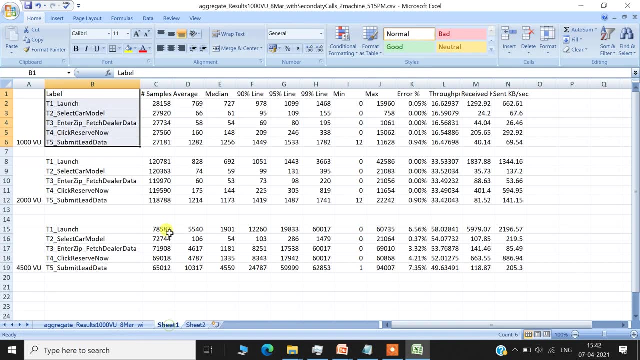 to use 90% time. So you can also use average. you can use 95%. I am going to use 90% time only. Most of the cases we use 90%. So what I am going to do is: first I am going to copy the 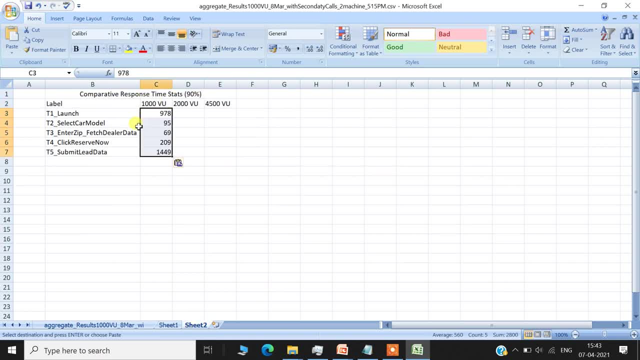 1000 user data copy in the 1000 view From 2000 also. I am going to copy that 90% line data. Similarly for 4500. I am going to copy this thing. I am also going to do one more thing. I am going. 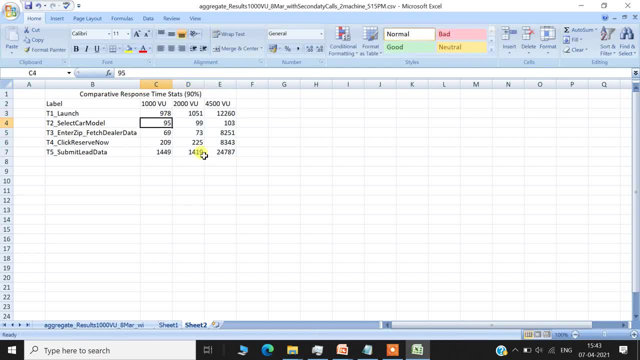 to Okay, so this, so now under. So one more thing which is very important here: the data, or the, by default the data that is generated by Jmeter, the unit is millisecond. So this 978 is millisecond, This, this data, is 920 millimeter. this unit is 300 millisecond And 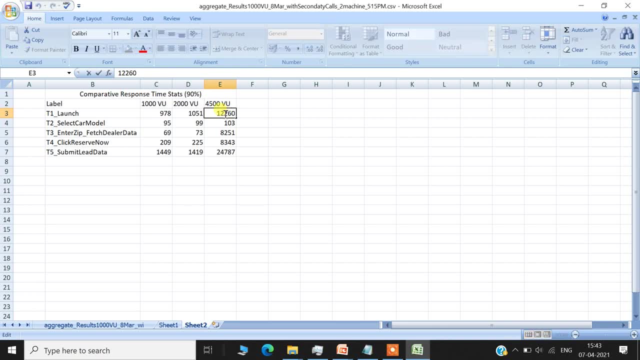 this unit is 600 milliseconds, so this one is 12.2 seconds or 12,000 milliseconds. so one more thing: what we can do is i am going to just copy this data here. i am going to add one formula, so here divided by 1000, so that 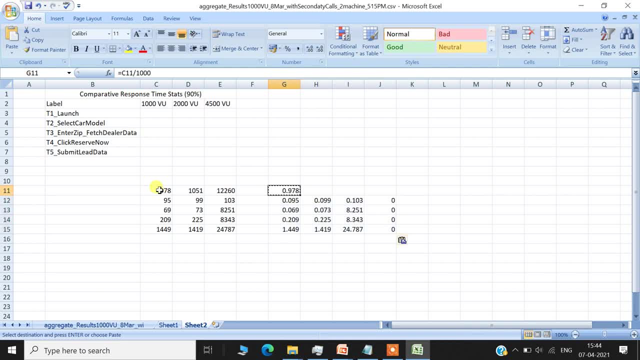 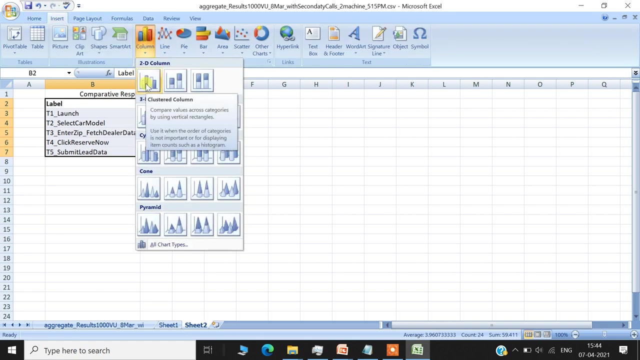 all the data gets converted into seconds, so just copy this, paste special values. so now i have the response time comparative data in seconds. what i am going to use is- i am going to create a chart for this. so how i am going to create. i just select this, insert, go to a column, first one, only 2d column here, if 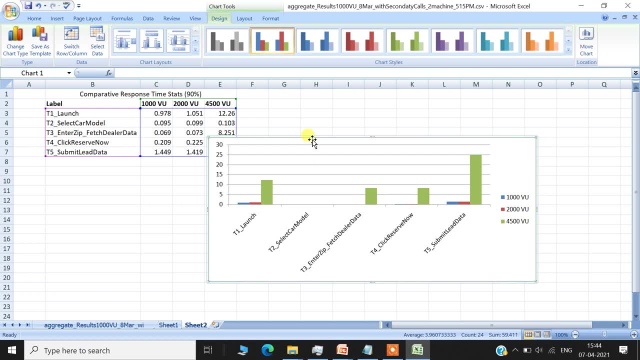 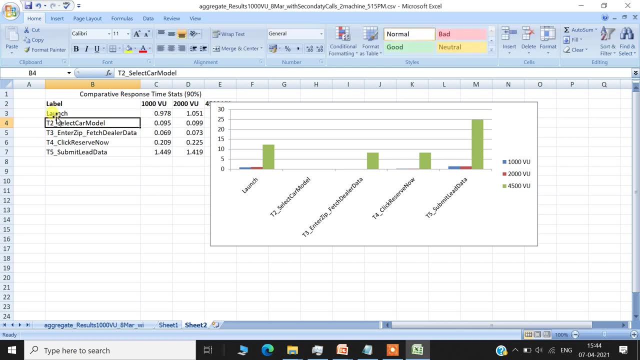 we see, we have the data. sometimes the names become too large, so we can also remove these t1, t2 while we are creating the chart. we can also delete these data or these names. so now, because the business team or the development team or the tech team would 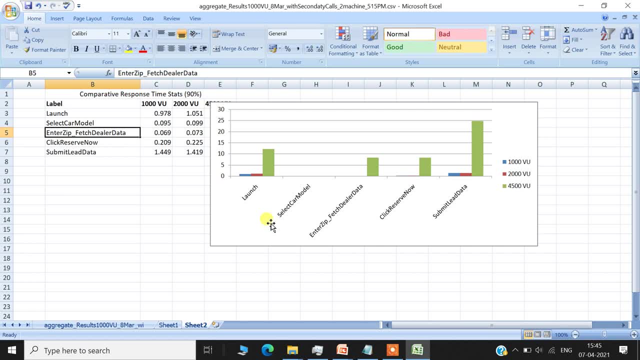 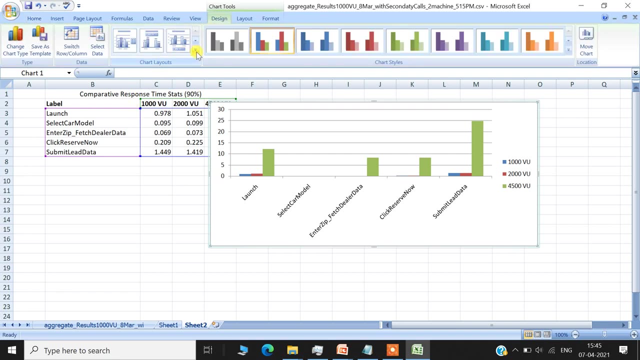 know these names, not the t1, t2, t3. so now we can see. this is the 1000 user results. i am also going to make some changes to this chart, so if i double click on here i also see chart layout. so i prefer this chart. 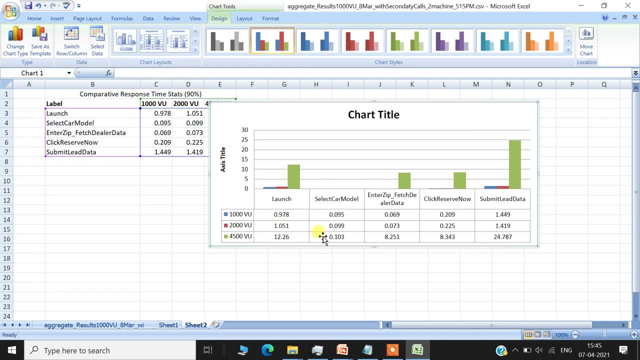 layout 5 where i can also see the time or the values that were there in my chart. so in the chart title i am going to share response. sorry, ninety percent response time statistics here. what is the? this is the response time in seconds bracket. so make sure that you give the unit, always give the unit. so here that. 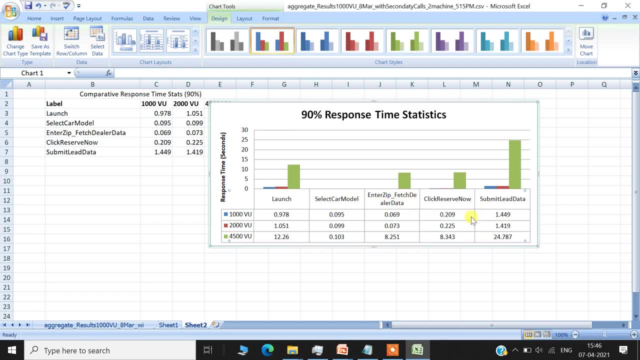 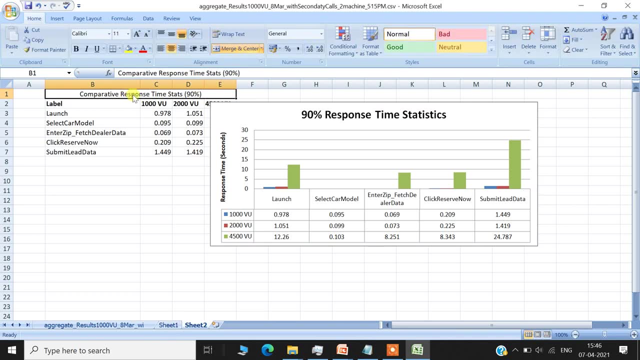 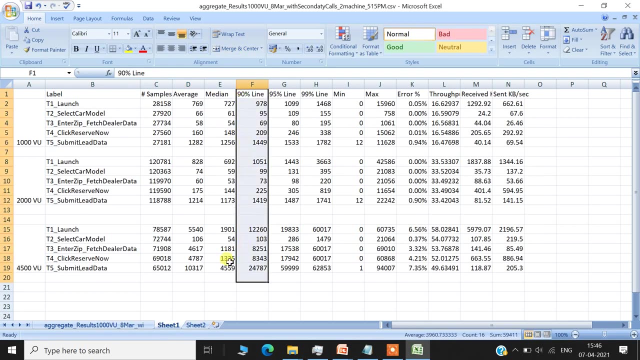 these are the transaction names: launch car model, select car model, these thing and corresponding response time. first stats that we are important stats are the response time. second important stat is: so let me just mark this one. so when we are going to use is response time comparison. second, we are going to share the samples or the number of 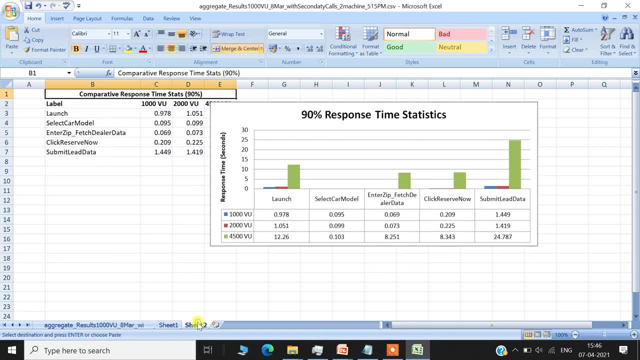 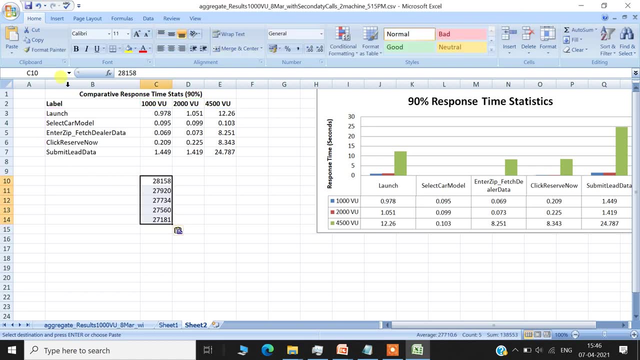 transactions that were made. so i'm going to create a similar table again. let me just move this chart here because the labels remain same, so I am going to copy the labels here. the load also remains same. so these are. these are the number of samples. let me insert one. 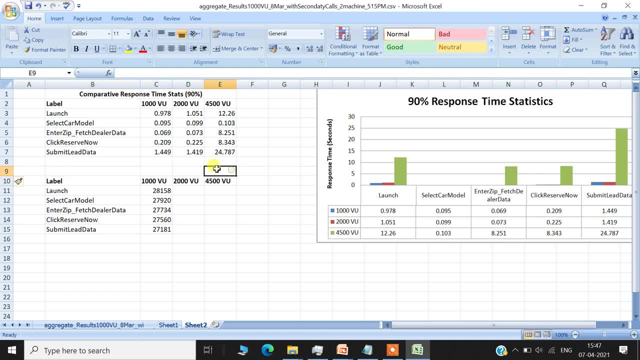 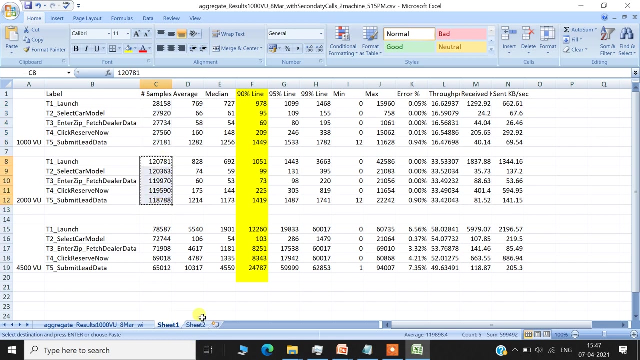 more file line, sorry. so here what we are going to see is comparative stats with respect to- oh sorry, come- transaction count. transaction count with respect to user load. so for 1000 user, these were the number of transaction that happened for 2000 users. I am again going to copy the same data for 4500. 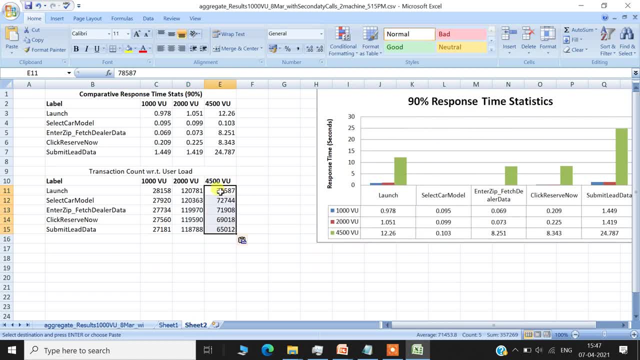 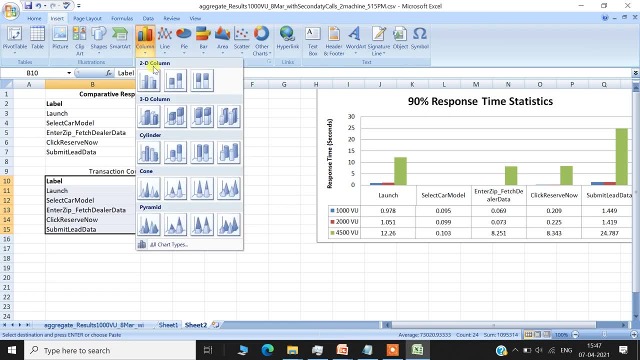 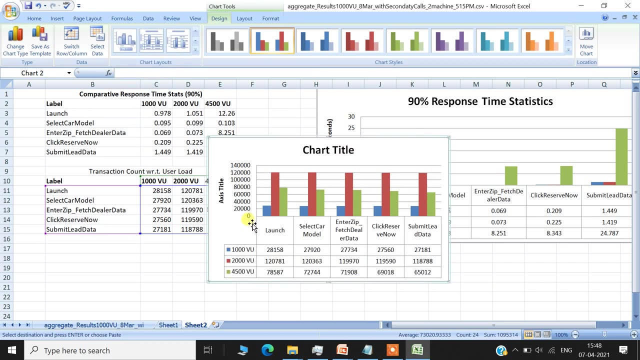 again, copy the same data again. I am going to create another chart here. so chart layout: I am again going to use that same table. find, change the name of the chart, title change, give this axis as the number of transactions and we can create so. so I am NOT going to change. so to save some time. 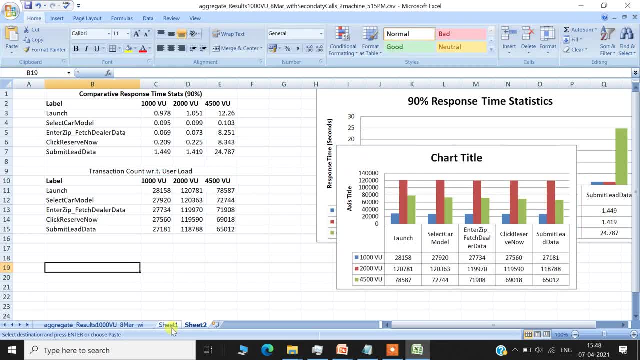 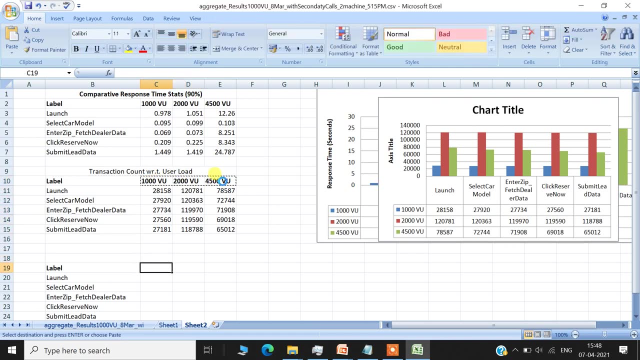 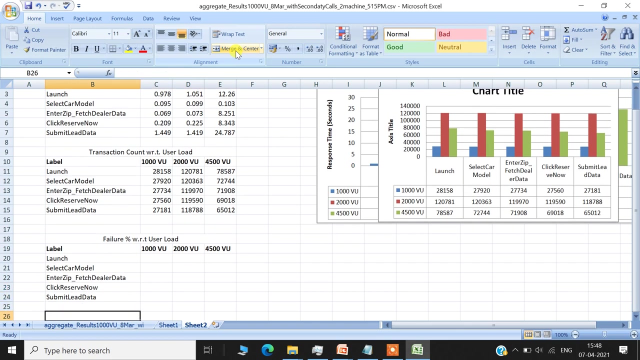 I am just going to keep it this way. only third important statistics is the failure statistics, so let us copy this again. create another table. I am going to move this here. so the third is failure percent with respect to user load. let's copy the failure percentage. this is the error percent for 1,000 users. 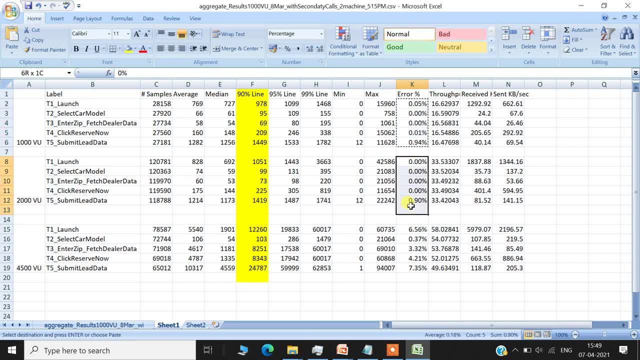 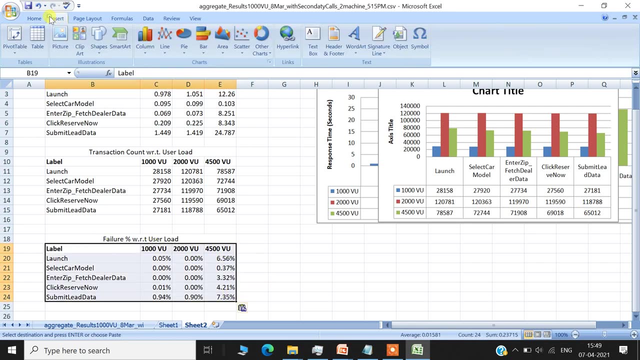 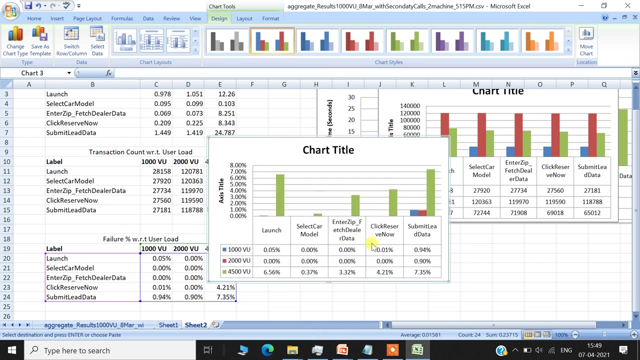 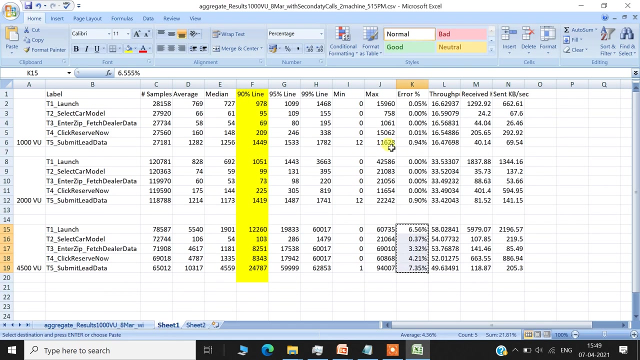 error percent for 2,000 view. error percent for 4,000 users. again the same steps. create a chart so you can see the data that is there, or the trends for the failure percent as well. so, to save some time, I am so these are the most important statistics that we should. 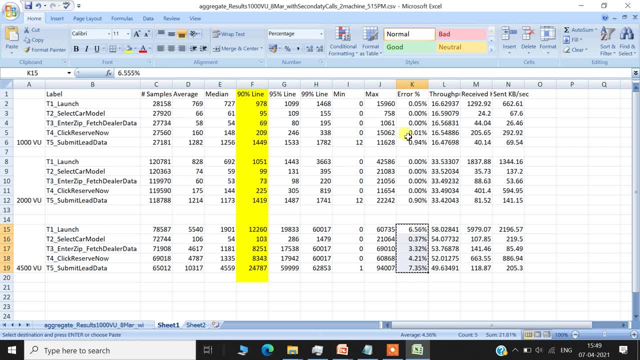 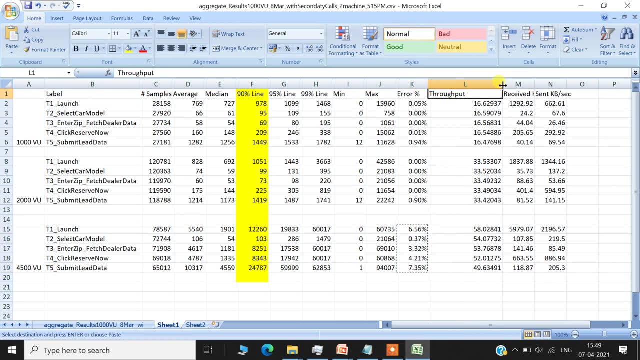 always share. this is going to give us the first-level idea or the important things about our test activities or the results. there are some situations where we would also require the throughput statistics, mostly in case of the API calls, etc. so we can do the same thing here if you use data that is used for a 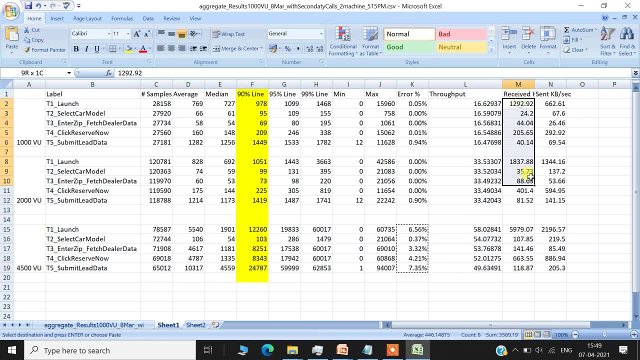 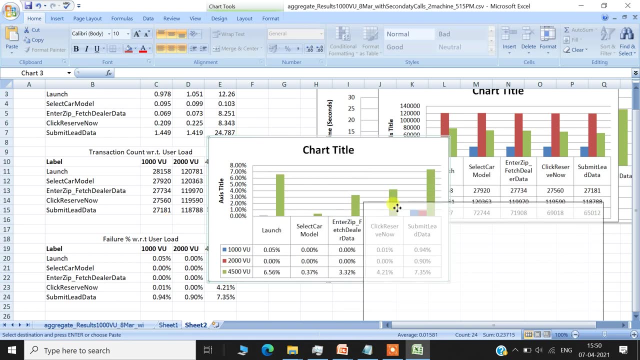 the same activity for throughput as well, data. i haven't seen being used this one, but there are very rare situations where we also use this. received or sent kb per second. but the important thing is the response time, failures and the number of transactions that happened during that interval. 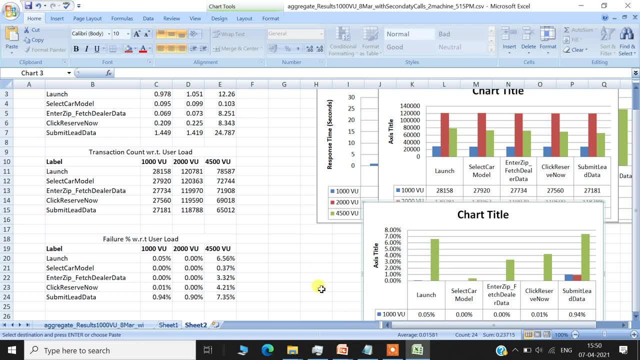 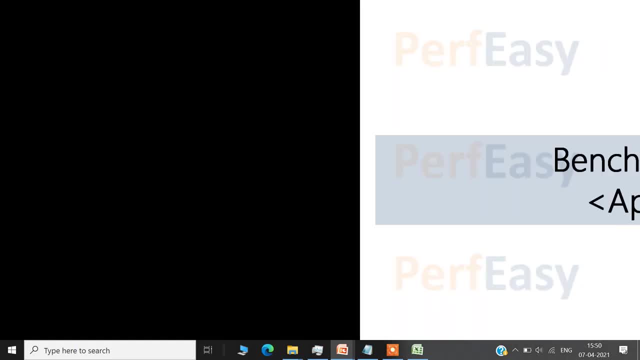 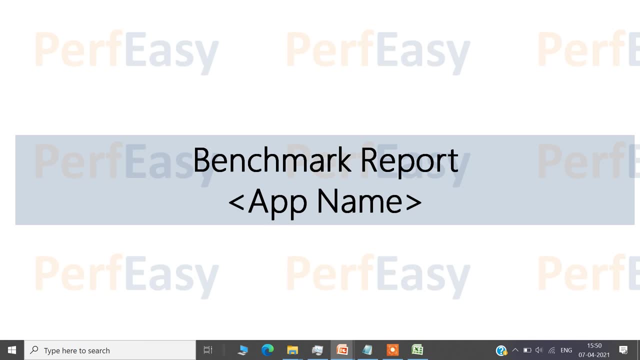 of time. now we have the charts ready, so i am going to go to my benchmark report. i am going to share you the kind of benchmark report. so here, the type of benchmark report that we share is: uh. this is the first uh page where we give the benchmark report application name or the client name. 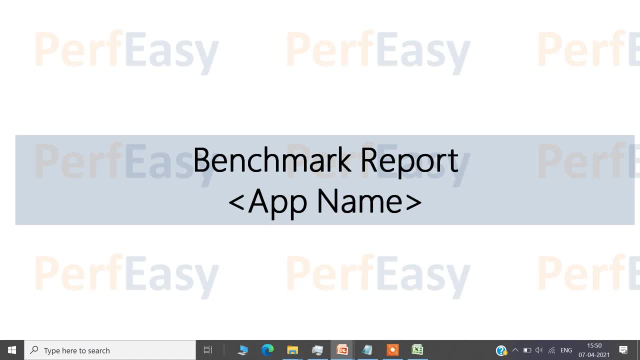 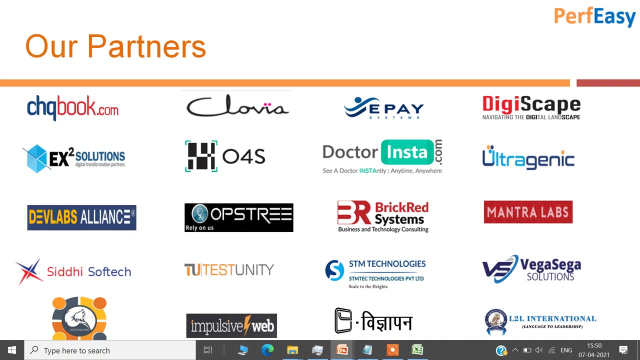 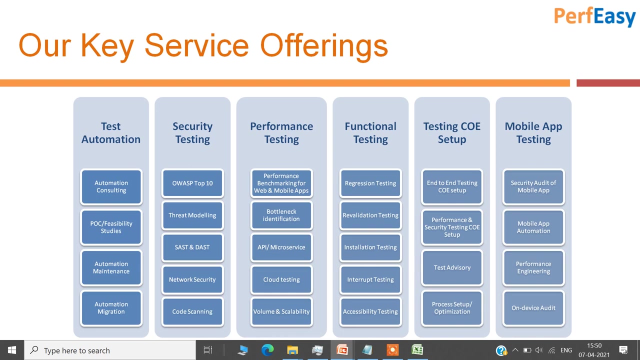 the relevant version number. also, where we did the testing uh give some introduction about ourselves as well. these are so from the perc easy perspective, which is a startup right now. uh, we have these uh served with these clients or serving some of the uh clients out of these. uh, these are the services that we are providing, the key services like test. 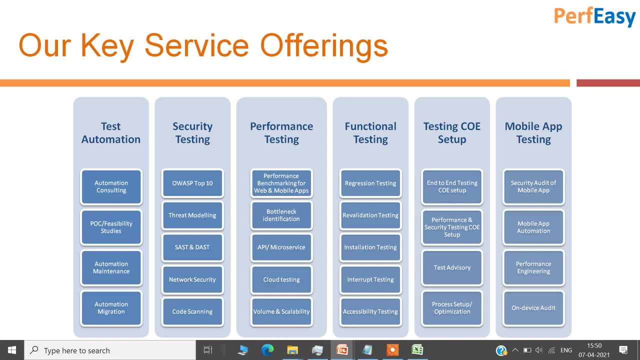 automation, security testing, performance testing, functional testing. we also do testing coe setup. as i uh, during my job as well, i have helped a lot of clients set up testing coes in and- important most importantly- the performance and security testing coes. we do the mobile app testing as well. 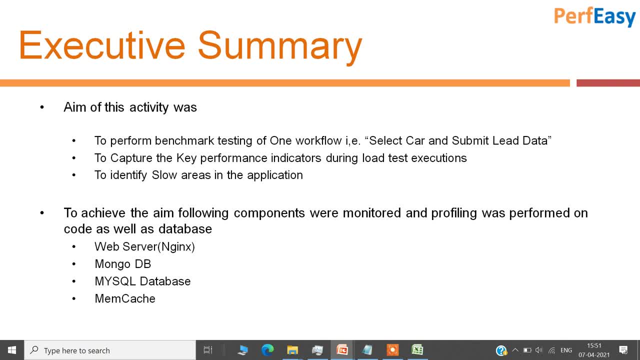 then we start with the executive summary in any report. so here this is the first step, or the first slide from the report, which is going to be: uh, give the representation to the uh business people as well as the technical people, that what was the aim of this activity and what are the different things. 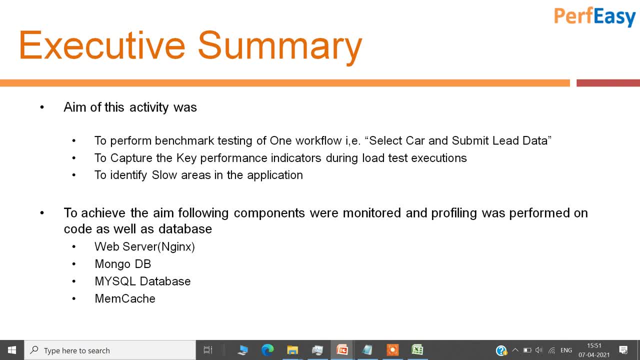 that we performed in this activity. so first step is: aim of the activity was so. here we performed a benchmark testing for one of the workflow, that is, select car and submit lead data. we also captured key performance indicators during the load test executions. here the aim was also to identify the 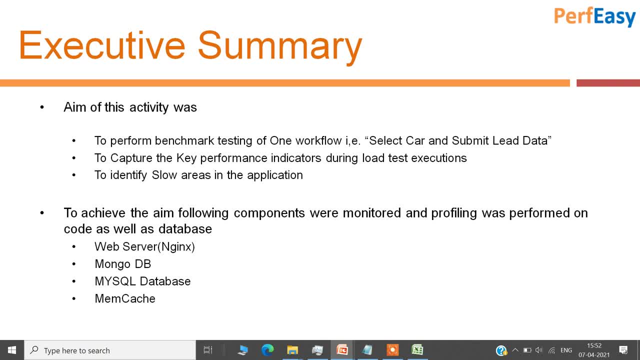 slow areas in the application. a slow area. so i can say that the lead data was very slow or the launch was taking a lot of time at a particular load. so those kind of trends are required in a benchmark testing activity. so here to achieve the aim, following components were monitored: like web server is engines mongodb. 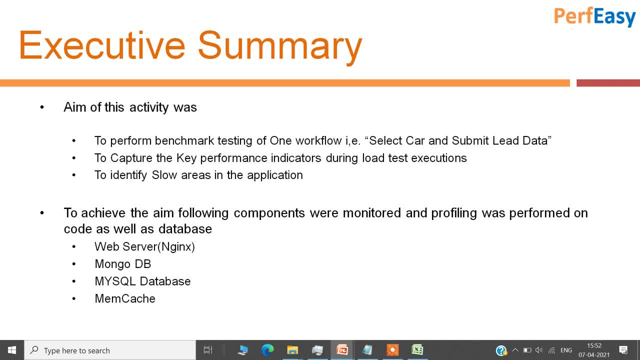 mysql database, memcache. so here we also mentioned that profiling was performed on the code as well as database, so this would be applicable in case uh, some back-end team is also monitoring the these components, or we are monitoring. so mostly this is done in a bottleneck identification. 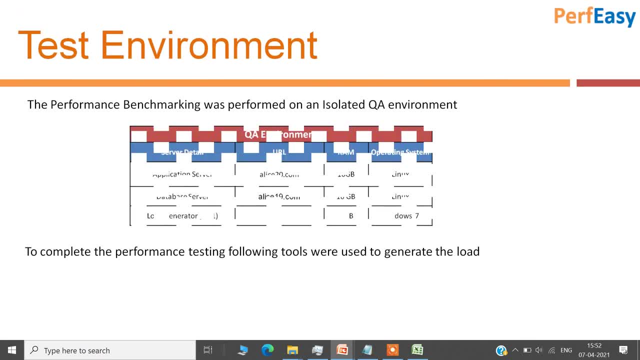 activity. so here this should not be present. then we uh detail out the test environment, because this is a very important thing. uh, most of the cases, the production. for example, a production has, let's say, 10 servers for that kind of 400 or 4500 or 10 000 user load. but the the type of or the kind of 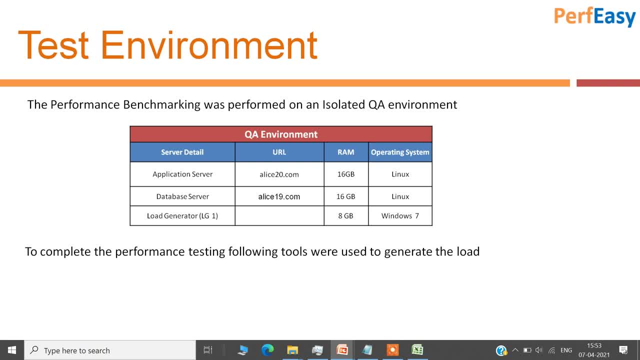 environment that we are provided for doing the performance testing is, most of the cases, is a scaled down version, so it is very important to make sure that we share the qa environment or the test environment. testing activities was performed with relevant information, like the operating system, the configuration, the ram, the number of cpus that were present, the type of machines that were available. 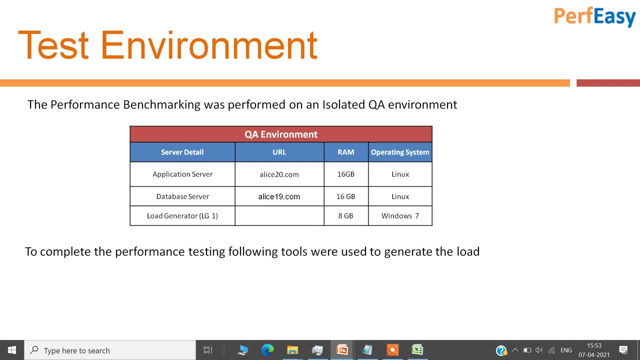 the number of components that were there. so we should always present there, or we should always mention the environment details here and we should also give what were the tools that we used to generate the load. so here only load was generated. so apache jmeter that was used, but there 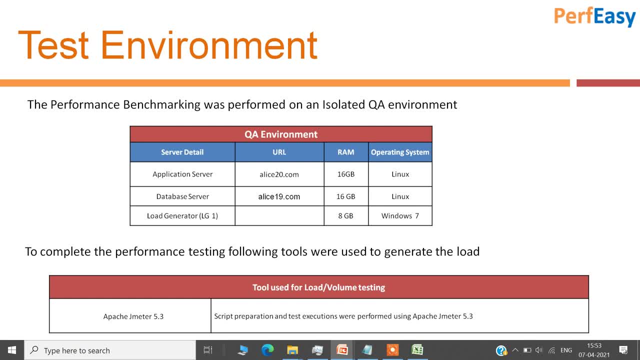 can be load. this can be new load. this can be any tool and if we were monitoring the server, for example a windows-based servers, we may be using a performant counters for monitoring the cpu. so we also mention the performance monitoring counters in windows utility, or we are using spotlight, or if 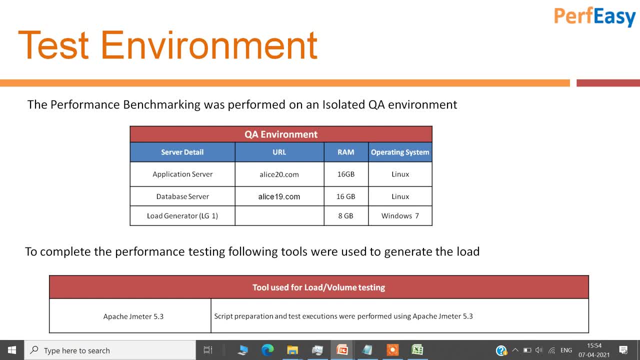 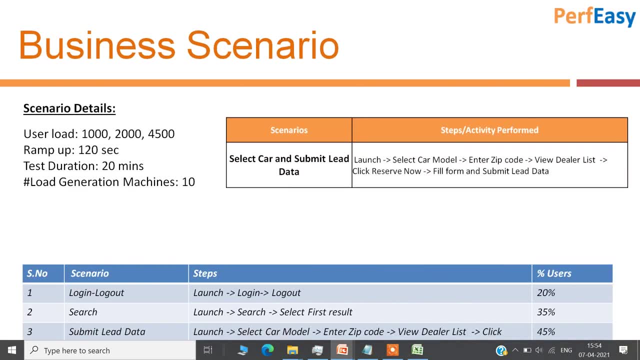 we are using app dynamics, new relic, apple gear, any apm tools that we should also mention that. another important thing is we should share what was the scenario that we tested, the results that we shared, so scenario, details. when we say so, how many users we ran? we ran 1000 user 2000 and 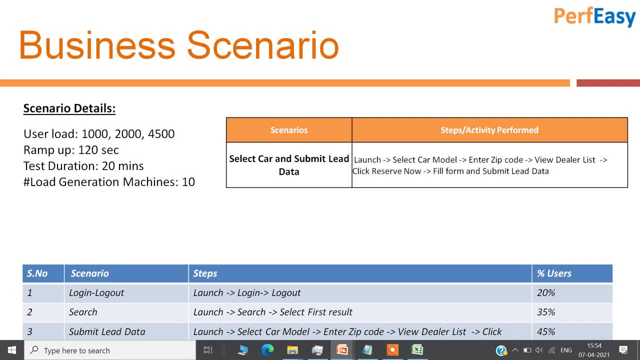 4500 users. the ramp up that we gave was 120 second here and the duration for this test was 20 minutes. so each test was ran for 20 minutes. each 1000 users test was performed for 20 minutes, 2000 for 20 minutes, 4500 for 20 minutes. the maximum number of load generator machines that we used were 10. 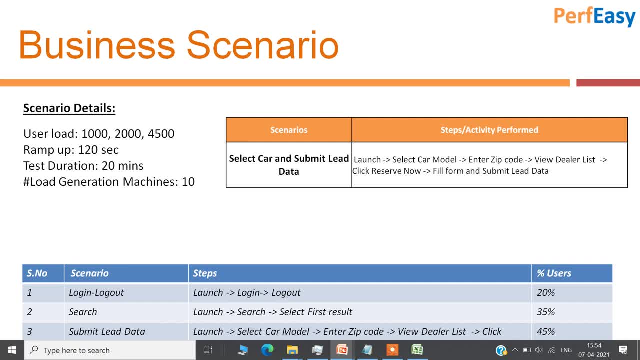 so one we used for control roller and nine were used for generating the load for the 4500 user load here. if you observe one thing now, everything remains same except the user load. so make sure that for when we are doing a comparison we should change only one factor at a time. here we are using, changing only the user. 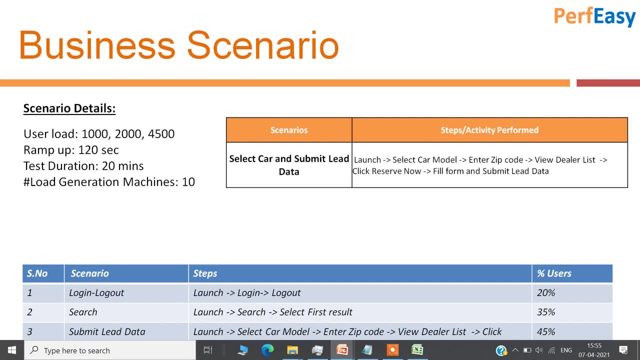 load. we keep on increasing the user load while we keep the ramp up as well as the test duration as same. in the right table we see the scenario: select car and submit lead data. this was the name of the scenario that we used and these are the steps that we were performing in our script. 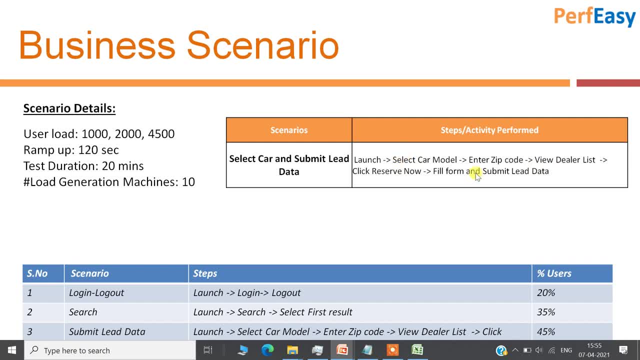 or the transaction that we had in our script. for your reference, i have also given you another table. so, in case of like, because this we have lesser time, so i used only one. uh uh, the workflow here. but in a real life situation we have multiple scripts. so here, if you see, the 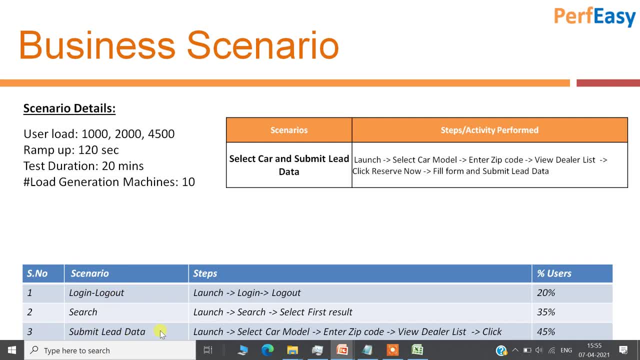 bottom table. so we have login, logout, search, submit data. so we have different steps for all these three scenarios, and the user load distribution is also shared. so depending on what kind of test we perform, we should give complete details of the business scenario that we used for running. so 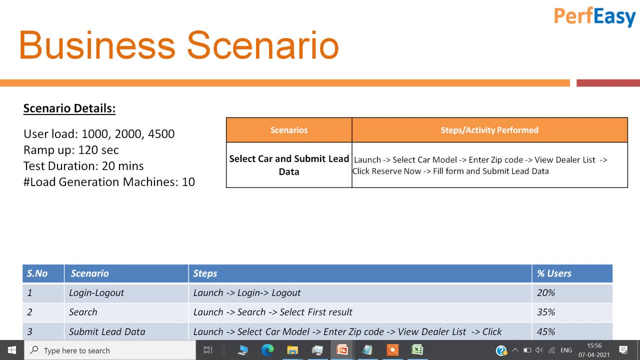 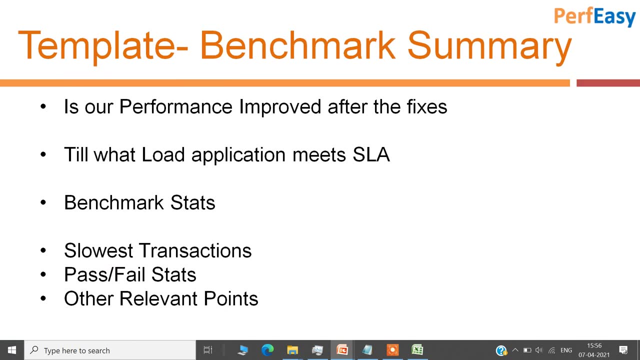 there will also be details about the endurance test, because in a benchmark we should also do benchmark test or a volume test or a spike test. so please mention all the scenarios that we tested so that it makes sense when we give the results. moving on, this is i am giving you some pin pointers, or 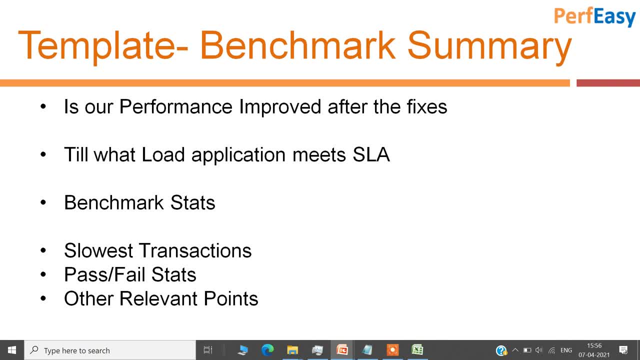 major points that we should also give in the benchmark summary. so after the scenario details, after the test environment details, after the executive summary, we should give the benchmark summary, which is going to be important for the business people. so mostly in a business, people are asking: is your application? so in case, this is the second round or the third round? so we 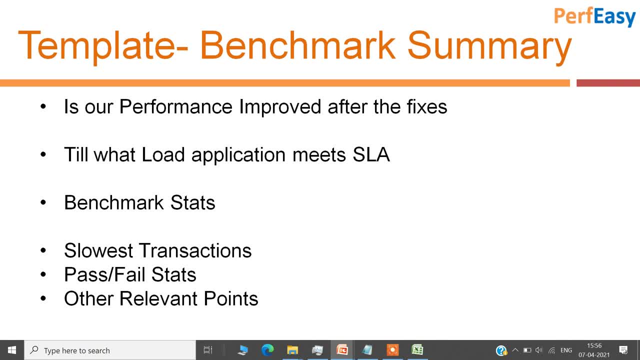 should also give some data that the from first round we have achieved five times the performance or no, with this build. the performance has decreased, uh decreased, or the performance has degraded. so we first step is always give if the performance impacts or the performance changes that were made. 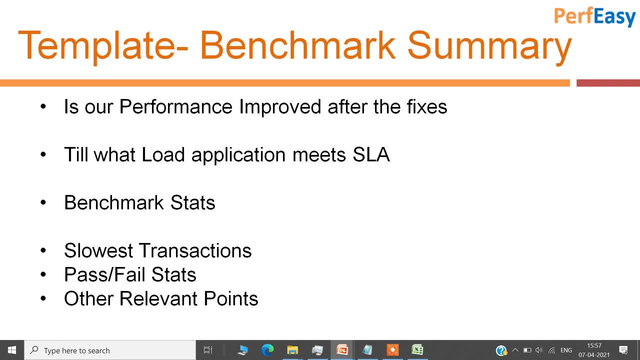 in the this build have positively impacted or negatively impacted. this information should be there. then the most important thing is till how much load my application is meeting my SLAs. for example, in our case the load up to two thousand user, the response times were okay. but at forty five hundred user the response times start getting very slow. we should give the. 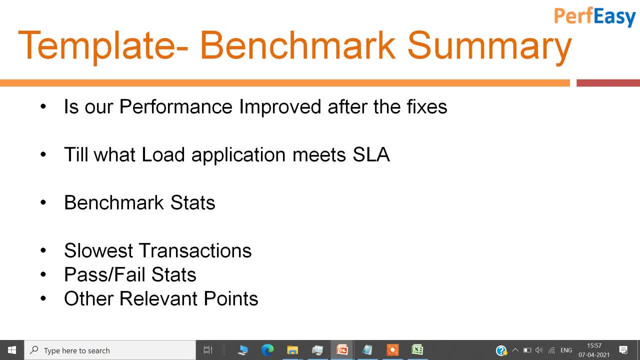 benchmark statistics. we should give some slow transactions which are the slowest pages that were opening. so here there can be a situation where we go into a little more details and we share the uh specifics for which request was taking most of the time, as well password statistics and other relevant point depending on the test you were performing. 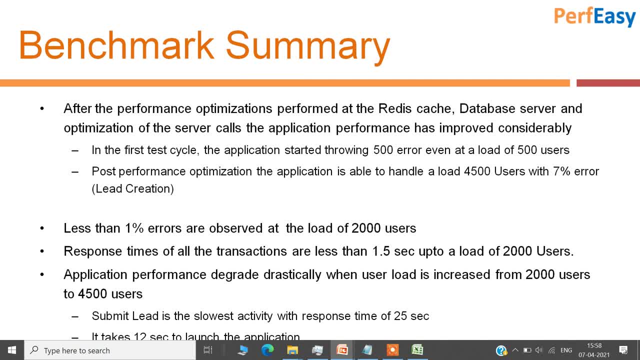 uh, let me share some data so that this information makes sense. so here first we have given after the- so this is the comparative data- is our performance improved? so here i am giving some reference. also after the performance optimizations at redis cache. so where we uh made the changes, redis cache was enhanced. the database server was also uh, uh uh modified, or the 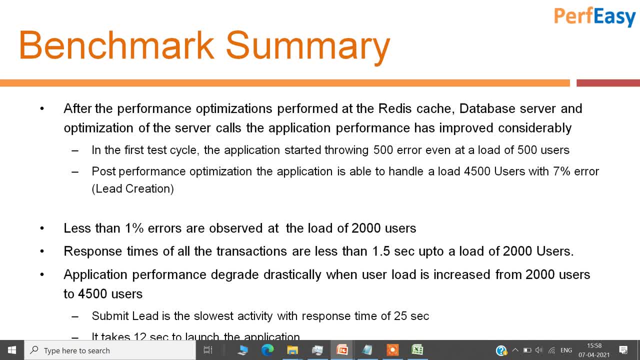 database queries were also modified. some optimizations on the server calls were also made. so based on that, we see the performance has improved considerably. when i say considerably, we should also give some statistic. in the first test cycle the application started throwing five hundred error when we were running only five hundred users. 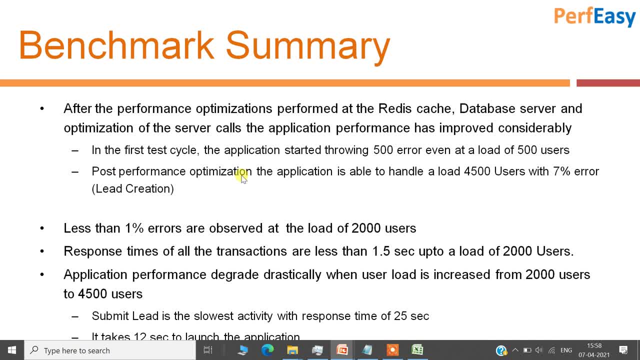 but after these changes were post performance optimization. now the application is able to handle a load up to 4500 users. that is nine times uh the performance. but still we are getting around seven percent errors during lead creation transition. so we are giving some statistic to uh make sure that, or to tell them that five year saying the performance has improved. or performance and come and decreded. we should. 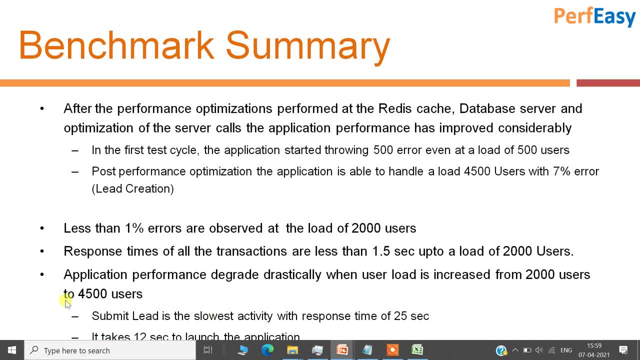 give statistics as well. then we talk about the current test cycle. is this build? in this build we see less than one percent error. up to 2000 users. the response time for all the transaction is less than 1.5 second. up to 2000. so here what we are telling is up to 2000 user the application. 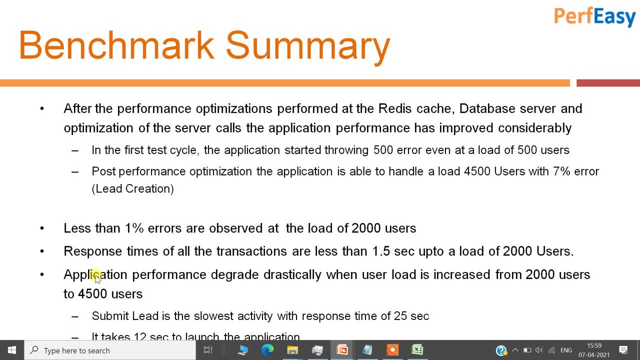 is fine. last point that we are sharing is the application performance degrades. oh, i'm sorry. the application performance degrade drastically when the user load is increased from 2000 user to 4500 user. so here the submit data or submit lead transaction is the slowest activity. 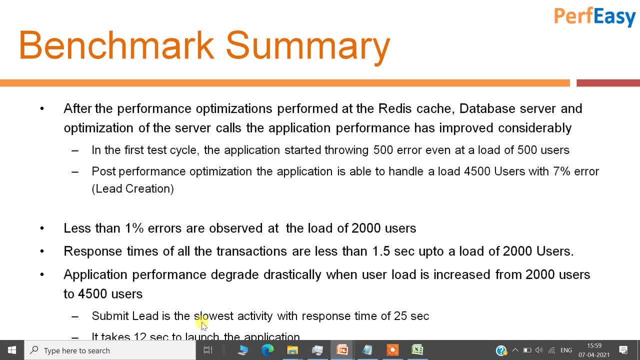 which goes up to 25 second and the 12 second is required or it takes 12 seconds to launch the application. so here we are giving some statistics that why we are saying at 4500 users the application gets 2.5 second. so here we are giving some statistics that why we are saying at 4500 users the application gets 2.5 second. 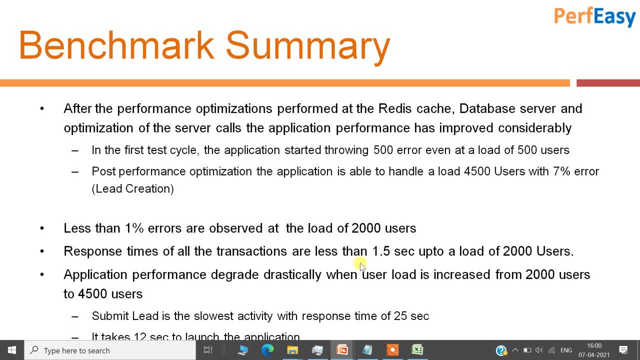 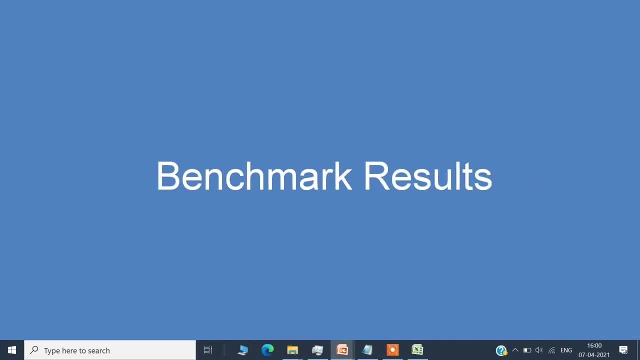 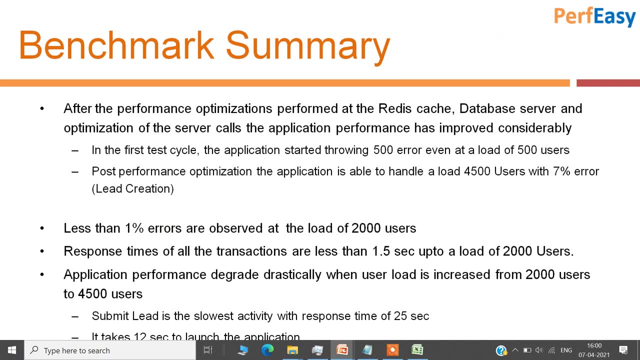 While for 2000 users the response time is always less than 1.5 seconds. Then we are going to share the benchmark results. So this till this point. we shared the environment details. We shared the tool details, the executive summary. what was the aim of the activity? 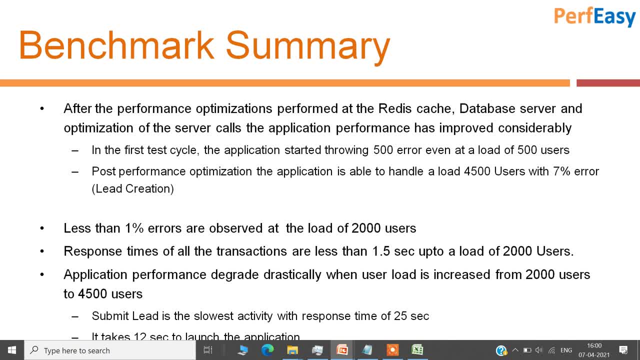 Then we spoke, also spoke about the test environment details, the scenarios that we tested. Here is the summary of the test or the observation that we captured by seeing those statistics, the charts, the response times, the failure. This is a summary of that result. 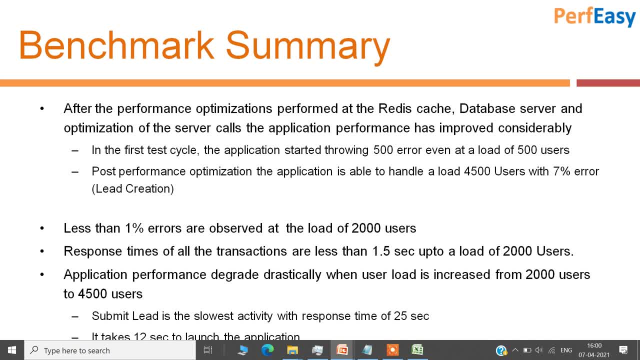 So for a business user, this slide is the most important thing. They are going to get this data. Then they will feel very happy that, yes, you have done the analysis and now you have pinpointed that this you go live till 2000. user. 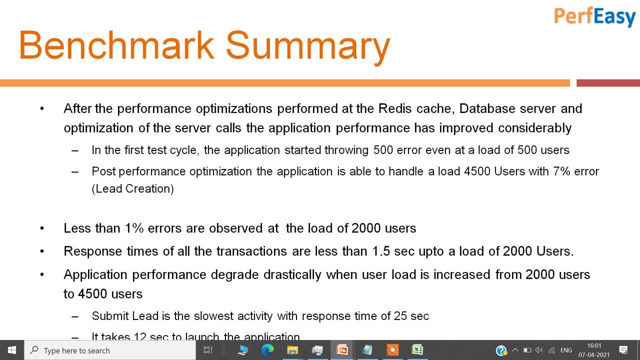 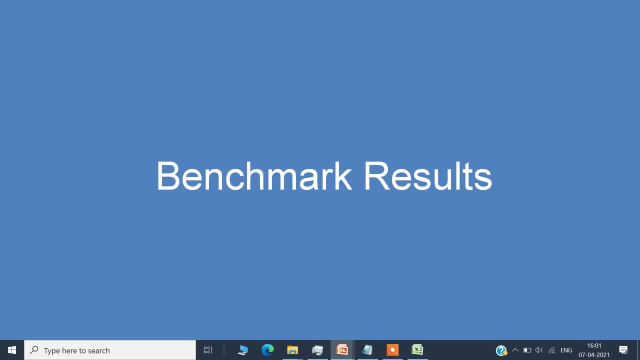 It is okay, But if you are targeting 4500 users, I am sorry, I am saying no, go live. So now we are also going to share the benchmark results here. This is going to be more important for- although it is important for business users as well. 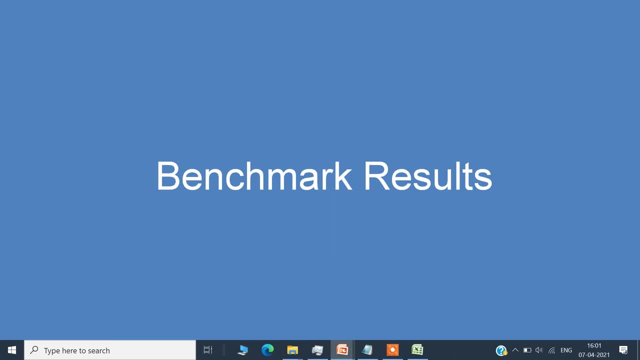 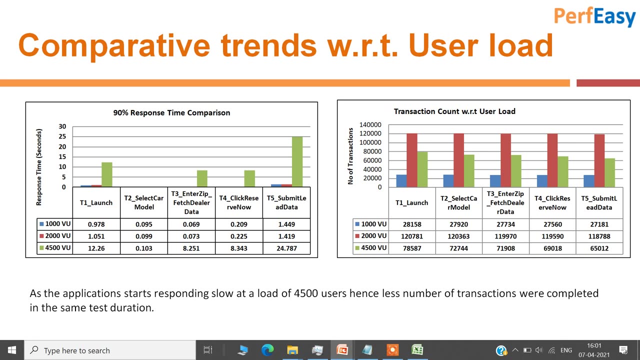 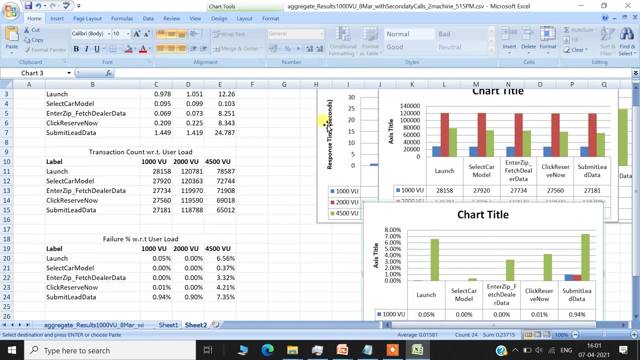 but more important for the technical perspective, the technical leaders or the development perspective, which can see why it is where it is getting slower. So here the same charts that I created I have copied here. So just copy paste The charts. how I copy, I just, for example, I copy this first one. 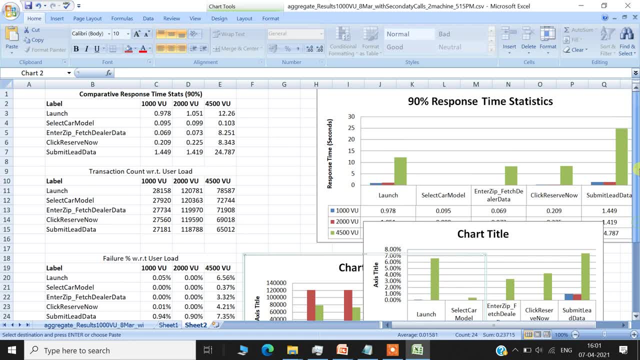 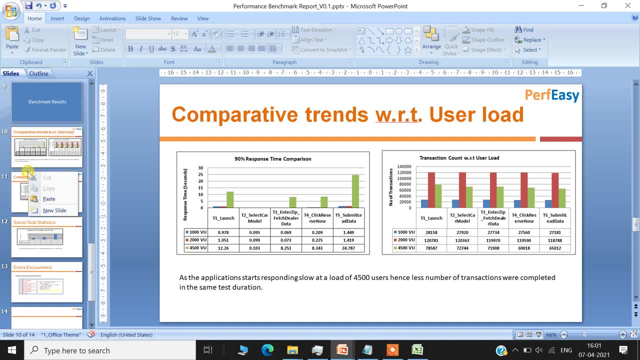 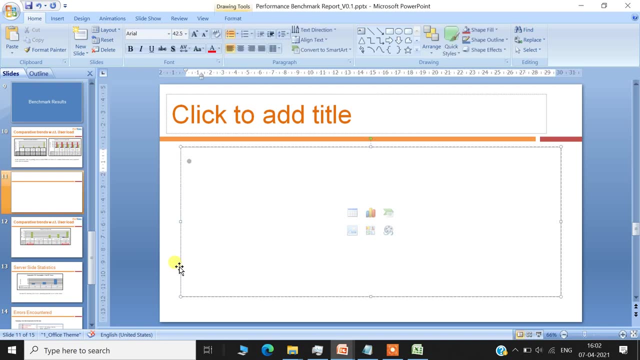 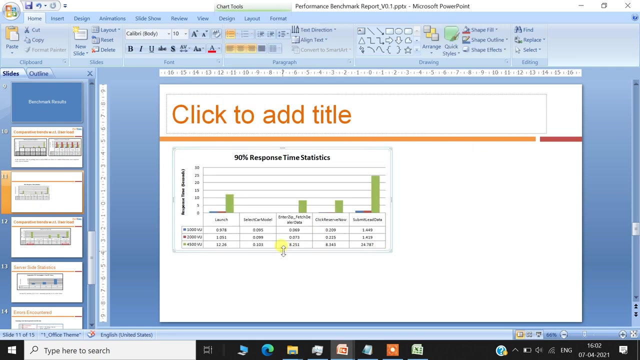 Let me move this one. So first one. for example, there's 90%, just control C. move to that way. Let me just create a new slide. Copy that slide, Copy that chart, And I can also do a bold here. 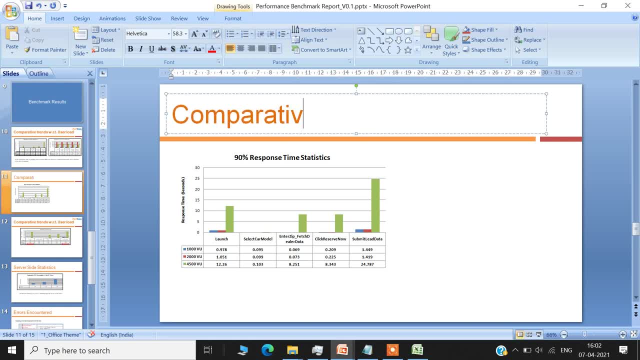 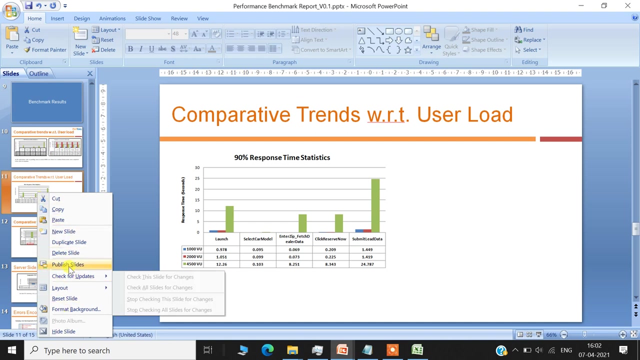 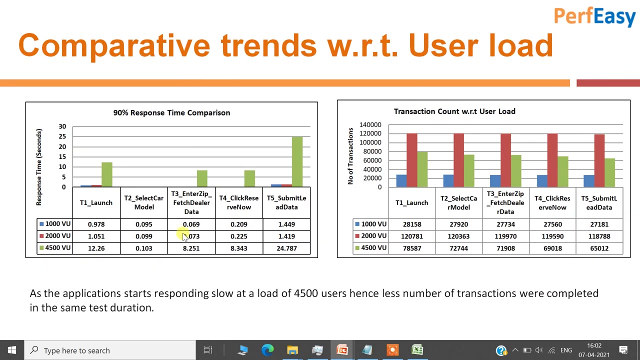 Give this comparative trends with respect to user load. sorry, just copy those charts here. So I have already done so. I am going to delete this so that we save some time. I do not think that copy is to be told So here. if you see the response time comparison, I have given transaction count with respect. 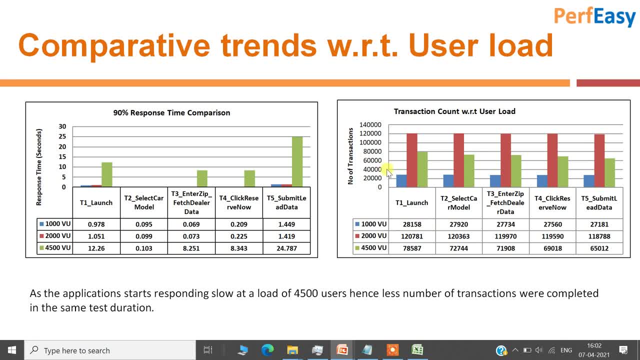 to user load. This is the number of samples. So here we also see. see, we should also give some observations here. If you see the bottom stats, as the application starts responding slow at a load of 4,500 users, hence lesser number of transactions were completed in the same duration. 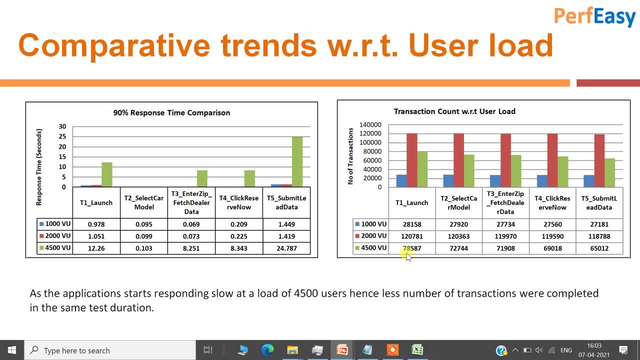 If you see now, Okay, For 2000 users we are making around 1,20,000 transactions for launch, While for 4500 users the number of transactions reduces to 78,000. So here the expectation was: with more users, we should be able to make more transactions. 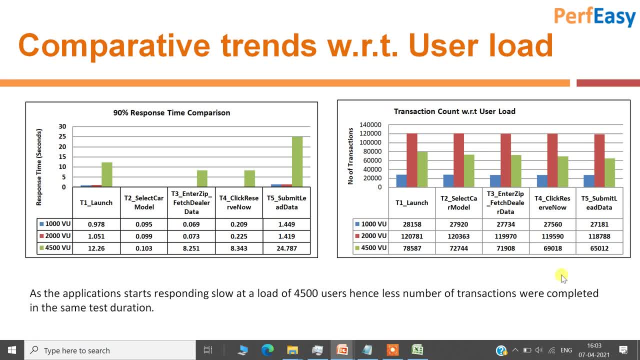 So why the same situation is not happening? The number of transactions is lesser for all the transactions Because, see the response time In 2000 users the response time is less than Maximum is 1.4 seconds. 0.2 seconds, 0.07 seconds. 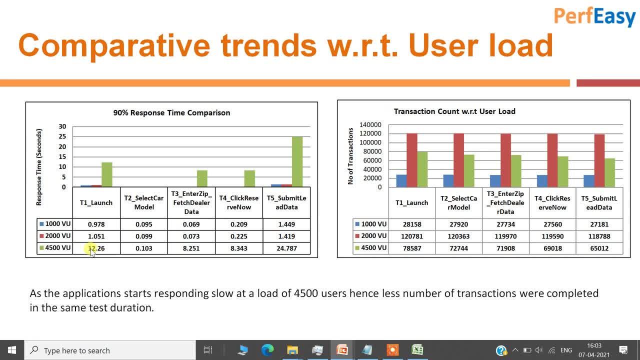 But in case of 4500 users the 1 second goes up to 12 seconds, So 12 times higher. So the number of transactions that could happen in the same interval, That is, the 20 minutes, would definitely be lesser. So 24 seconds for the submit lead. 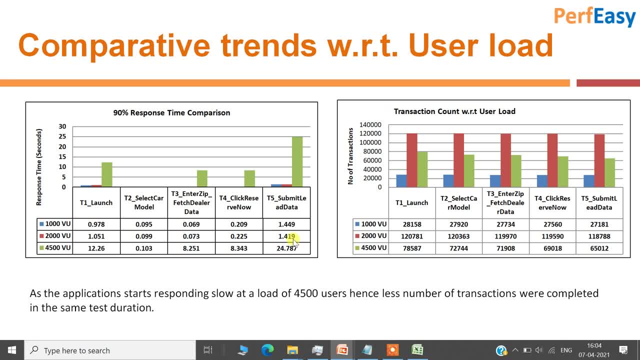 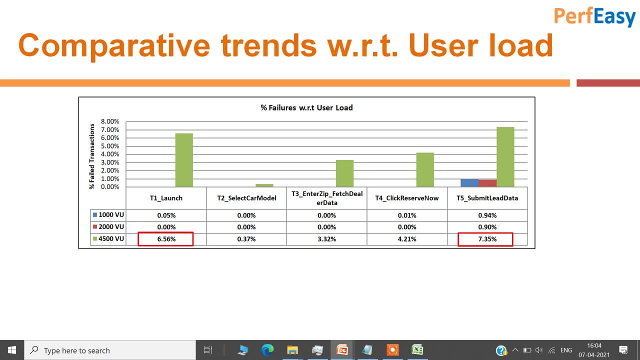 While for 2000 users it was only 1.4 seconds. So we are making around 1,20,000 transactions, So we should give these kind of observations as well. This is very important thing. Next I have shared is comparative trends with respect to user load. 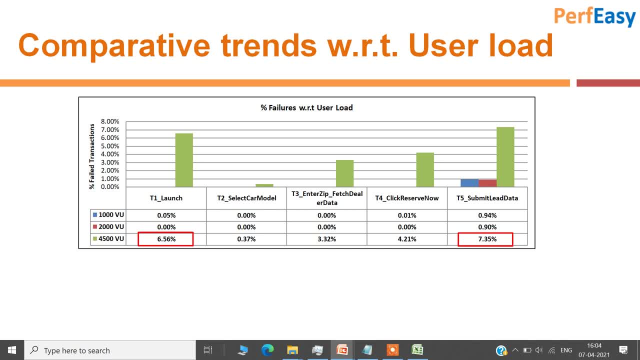 The number of failures or the percentage of failures that were captured. So here we see around 0.05%- 0.9%. So in most of the cases it is okay to have around 1 or 2% failures. But once we so in this application when we decided 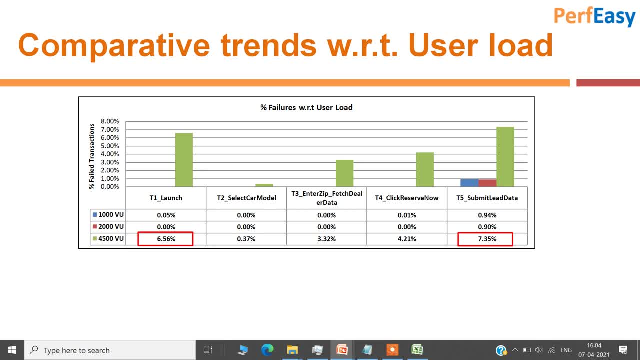 5% failures is will be our failure criteria. So here I have also marked these red color marks So that I can share. show that these are the transactions Where the failure percentage was higher than 6% or the 5%. sorry, 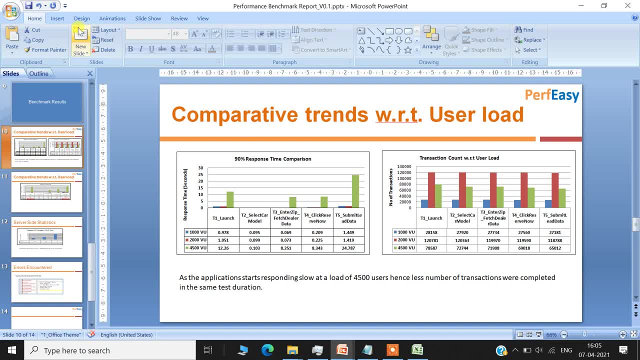 How I have done is: let me show you that. So here also, if I see now, So that the response time should also be marked this way. So what I am going to do is: I am going to do this, I am going to select this rectangle from here. 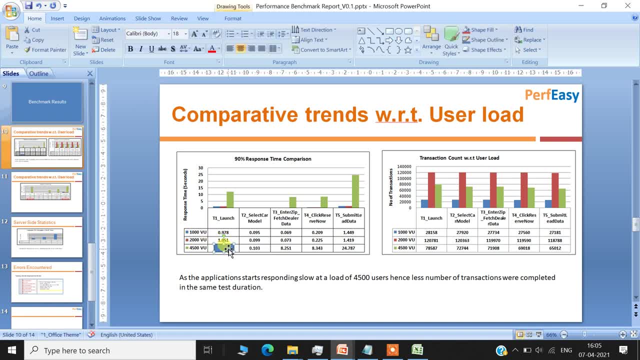 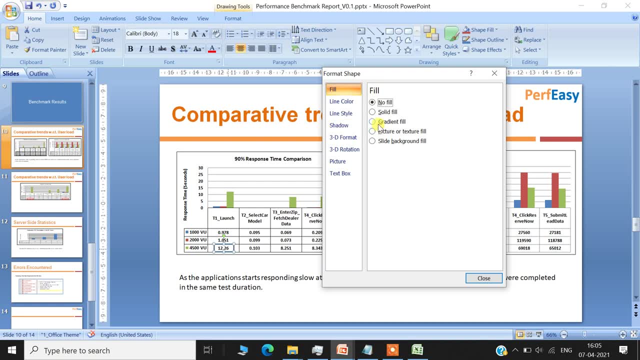 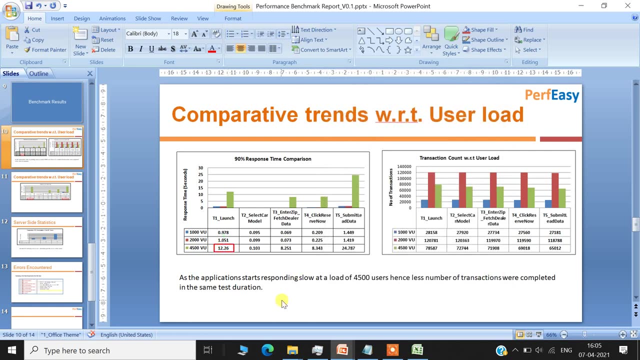 And I am going to mark this 12 seconds. Just right click format shape. No fail I need, because I am going to just mark Line color. I am going to give as red Close. So if you see this, 12 seconds now is also marked. 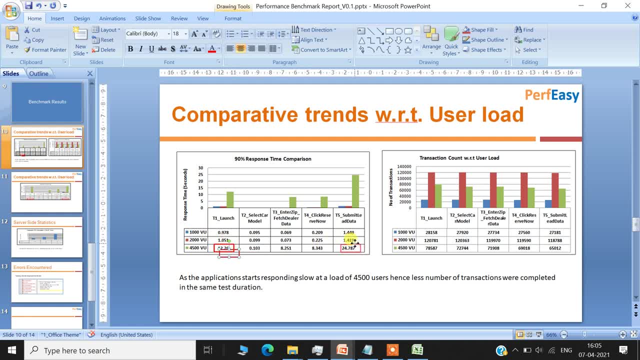 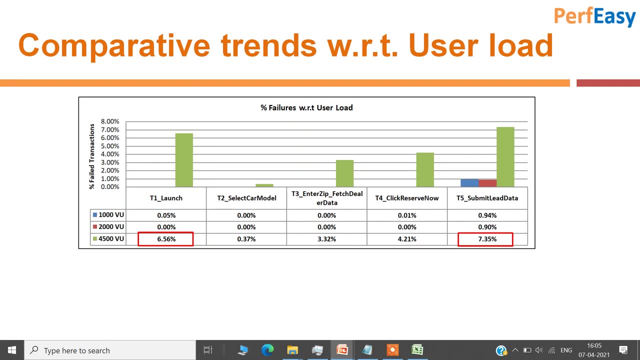 So when I share this report, I also just copy paste to the transactions Which are slow. So I am marking the transactions which are more than 10 seconds. So here. so SLA was 10 seconds for the response time, While for failure percentage our SLA was 5%. 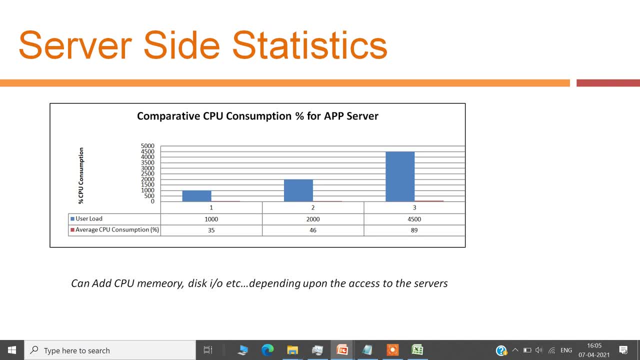 So here, as I was saying, if someone Is also monitoring the server side sets like CPU, memory, network, DiskIO, So we should also these kinds of charts here as well. For example, they are here. I am showing that 1000 users, 35% is here. 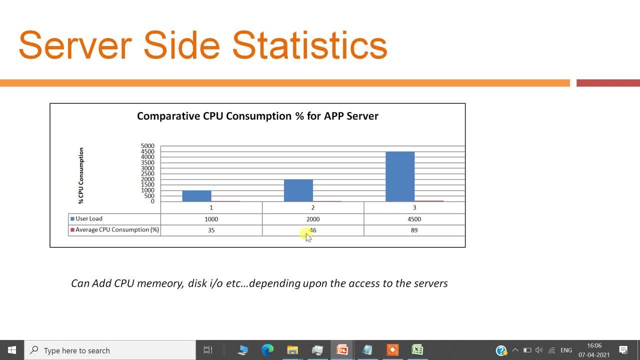 CPU consumption was on an average was happening for 2000 users. around 46% CPU consumption was happening for 4500 user. we saw 89% CPU consumption on the app server side. so similarly we can capture the statistics from the server side and share this. I will show you some better stats, some share, some in the 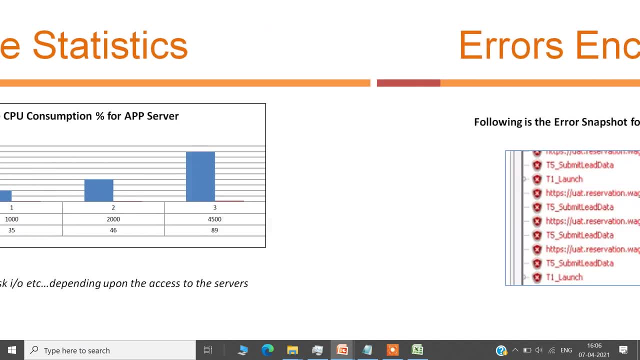 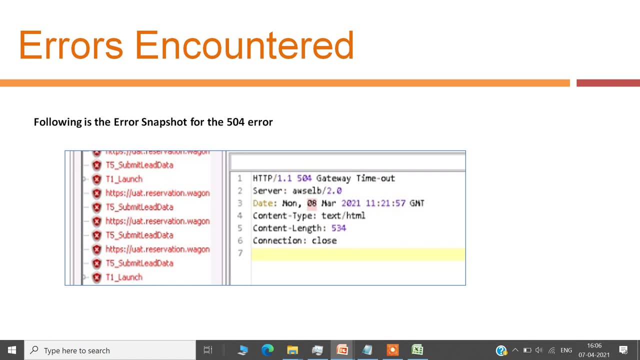 bottleneck identification report. so please stay with me. we should also share when I say that 6%, 7%, 5% failures were happening. so what was a failure? so we should also share that: screen shots for the failures, the error details that we were observing on the J meter and while we were running the test. we would also 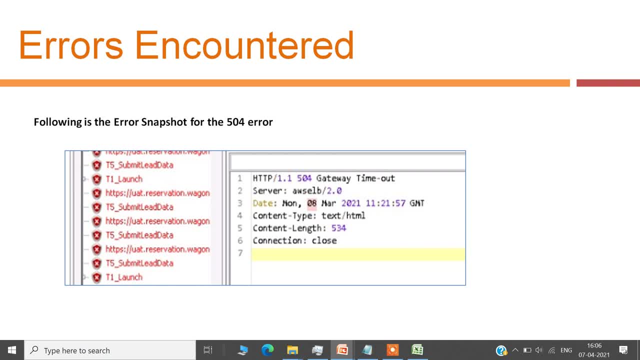 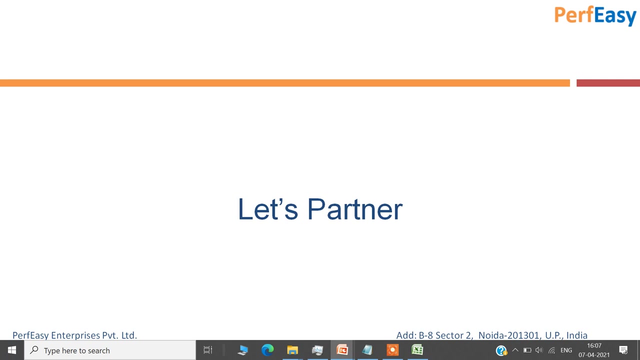 be running the application manually and we should share the men was relevant manually- the snapshot that we taken here also. so here we were getting 500 error a in the all that wherever failures we were getting. so i have shared one snapshot only, which was 504 gateway timeout. so let's partner is a end slide. thank you is a slide here, so this: 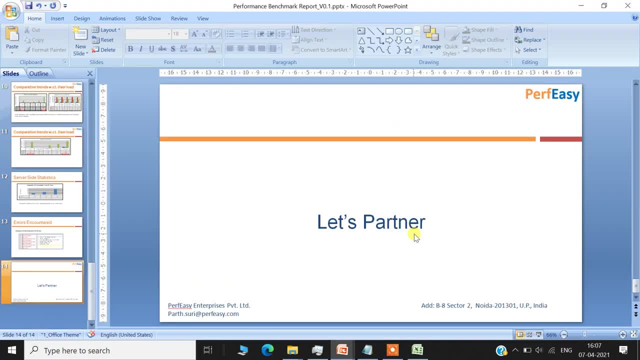 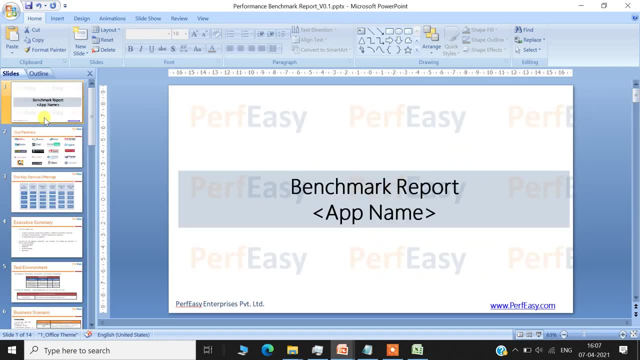 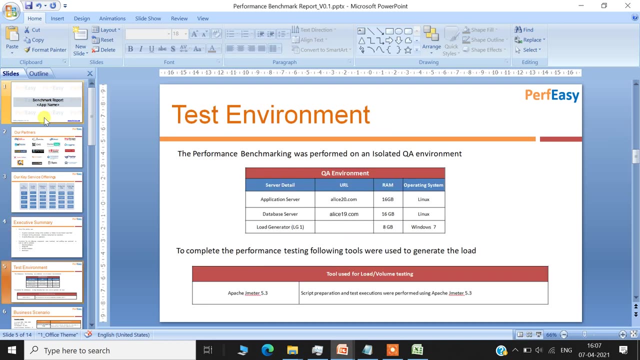 is the benchmark report that we share with our clients, so i hope this is a very helpful situation. let me just quickly go through all the slides again. quickly so: executive summary, where we mentioned the aim of the activity and what were the things that we monitored. then we spoke about 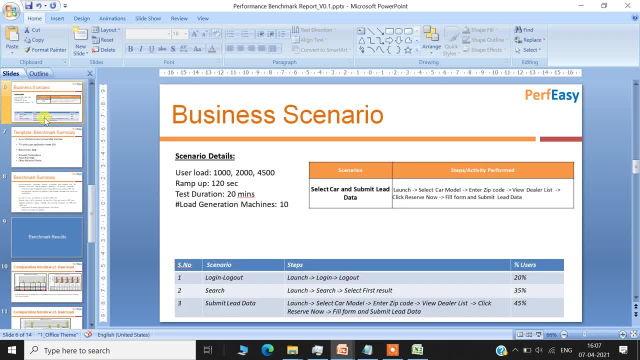 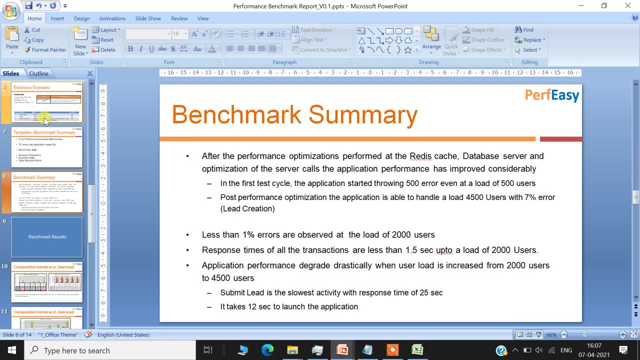 the test environment details. then we spoke about the business scenarios. then we spoke about the bench. we gave the benchmark summary. this is for the more importantly, for the business people, so that we are giving actionable item, so so that 2000 user- okay, 4500 users- no, go live. 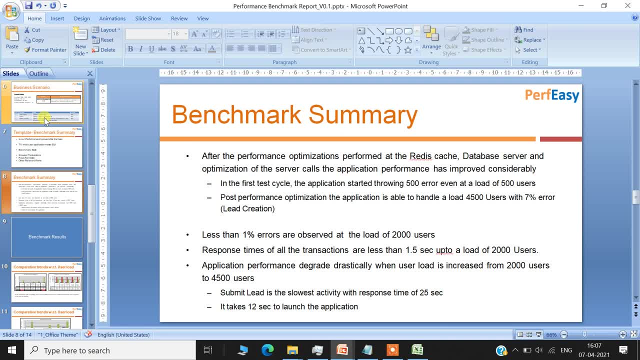 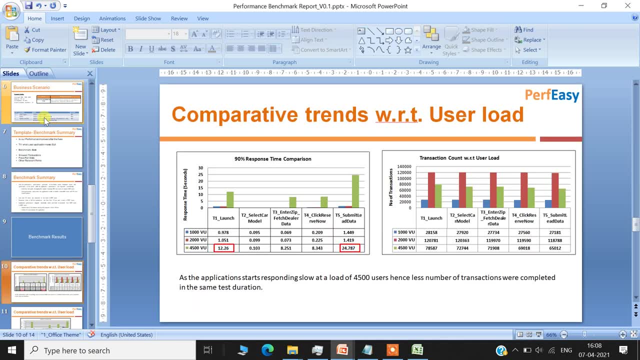 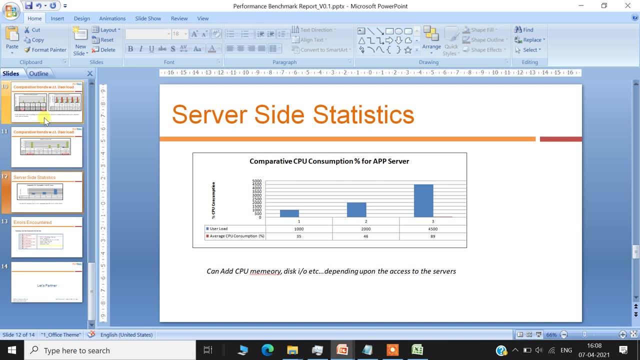 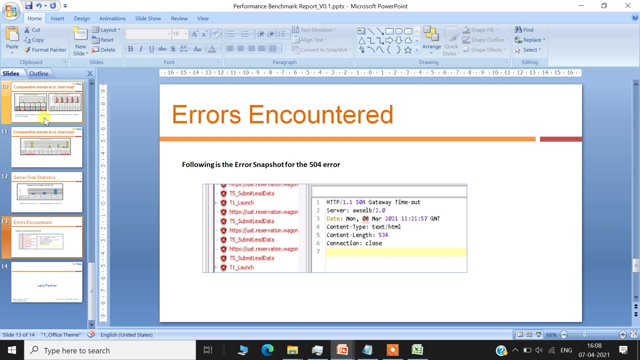 for if you have to do the optimizations, go for now 4500 user, so those kind of actionable items are here. then we shared some statistics from the benchmark data: the response time statistics, the transaction statistics, the failure statistics, the server side statistics, the cpu memory network, these kind of statistics, and then the last error details. 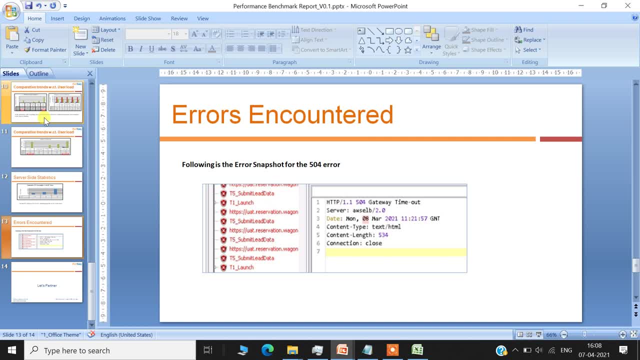 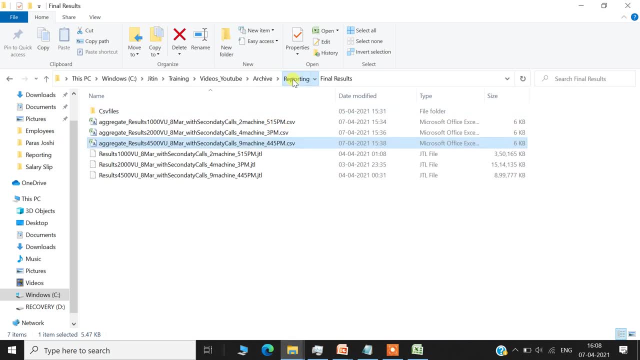 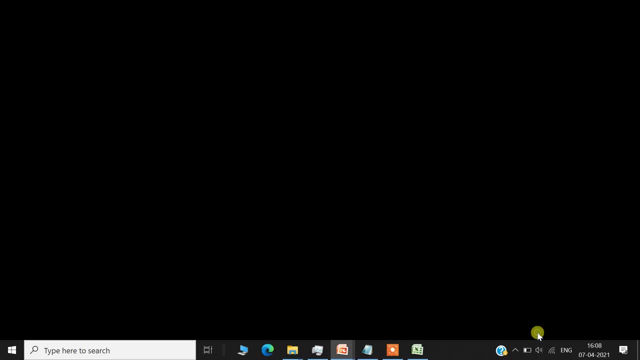 what were the errors that we captured. i hope this helped, so now let me also share you, as i promised initially, let me also share you a sample performance bottleneck identification report that we share with our clients. this is one of the example. uh this: the data may vary depending on what kind of activity we have. we are being 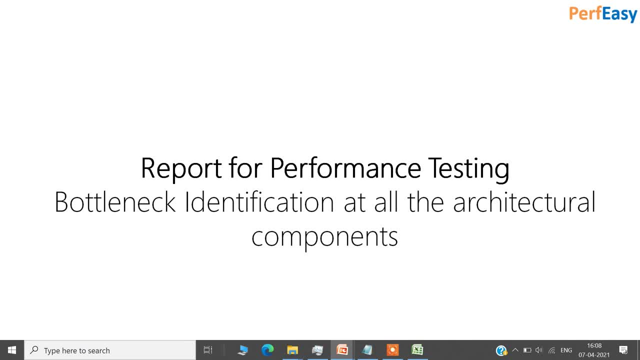 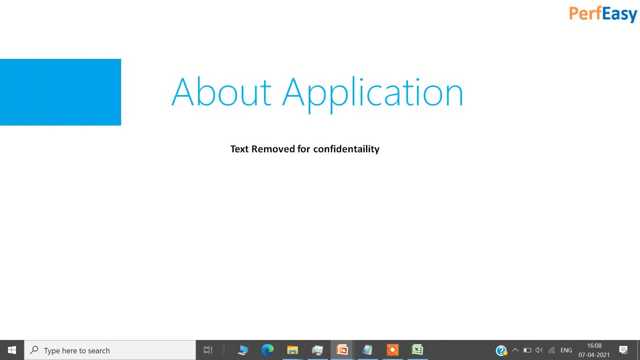 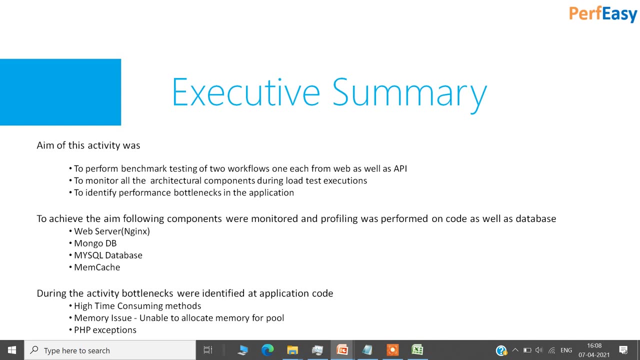 doing so. this is a performance testing where bottleneck identification and all the architectural components was performed. so here, first we gave some details about the application. so we have removed this because this was a client information result. so next is the same executive summary: what was the aim of the activity for? 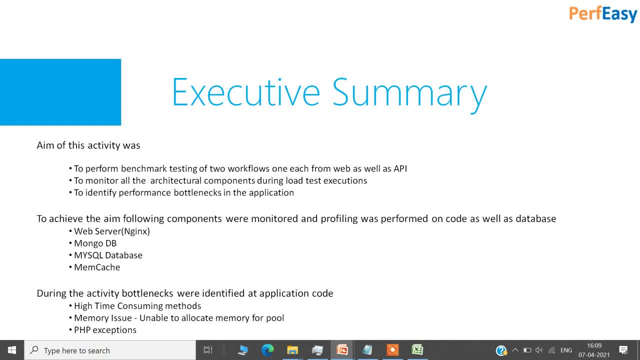 example, the two workflows, one from web and one for from apis, were tested. we monitored the all architectural component during the test executions. we aim was to identify performance bottlenecks in the application here. this is the next point. that is the aim. achieve the aim following: components was monitored and profiling was performed on code as well as database. so 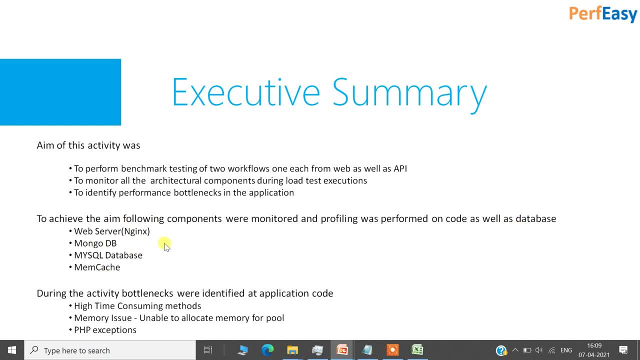 these were the database and the architecture level component that were present. we identified the bottlenecks at code level where the high time consuming methods were identified, some memory issues were identified on the code and some php exceptions were also identified. next, we also shared our approach. first phase, we did some application benchmarking. 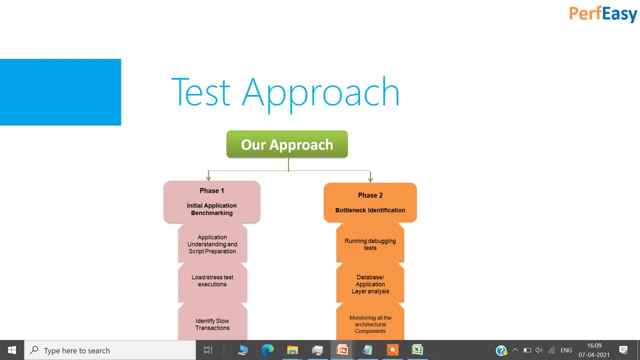 where we identified how much load application is able to sustain, so that we can give a comparative statistics after the fixes. because in first test we knew that 500 users, 500 uh exceptions were coming. so, uh, in the next round we we did a 500 user- uh comparison and now, yes, that passed. then. 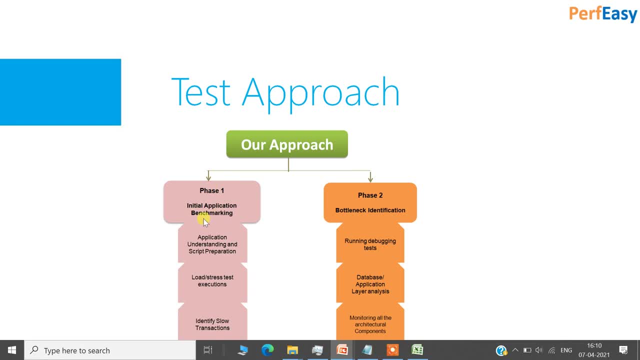 only we moved on to the next step. so phase one is initial performance benchmarking and this phase two is bottleneck identification, uh activity, where we did some debugging tests. we monitored the database and the application layers. all the components were monitored during the load test executions. next is the environment detail. we i already spoke, so here i am also giving you. 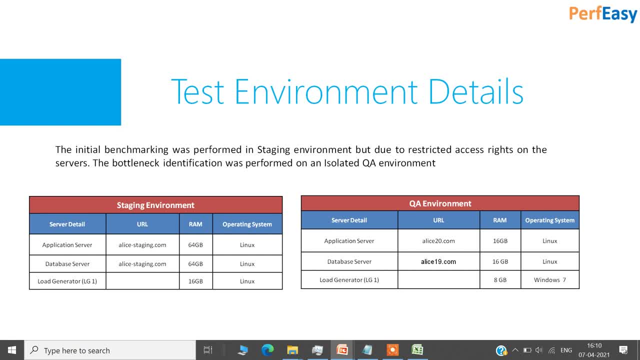 two kinds of uh, because initial benchmarking we performed on staging environment but there were some restrictions as we could not get the server access. so the bottleneck identification we uh were able to perform on the qa environment only. so we that activity was performed on two server set of environment. so both the environment details are given here. 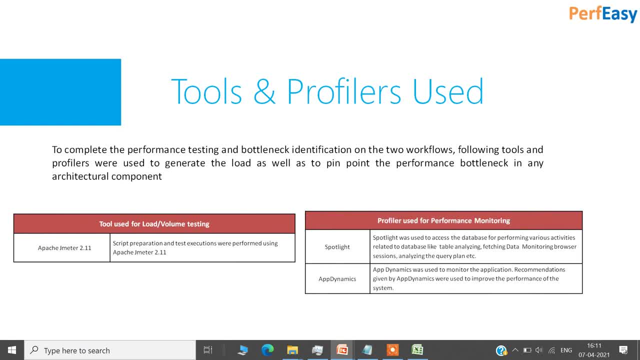 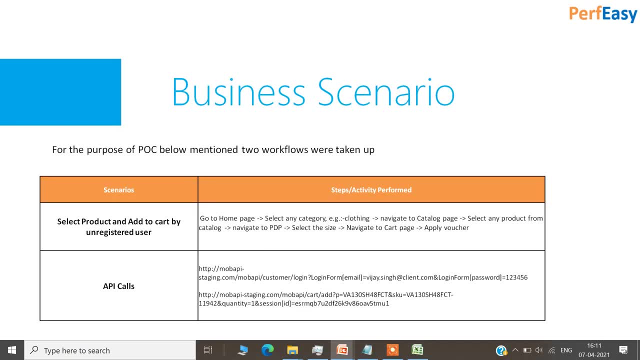 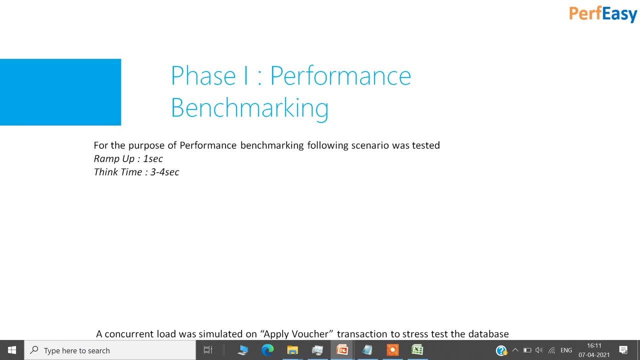 same the tools and the profilers. here we used app dynamics and the spotlight, so the tools that we used have mentioned business scenarios that we use. so now we are going to give the performance benchmarking data. the phase one performance benchmarking: we ran a test for uh one. second ramp up with three to four second think time. we ran the 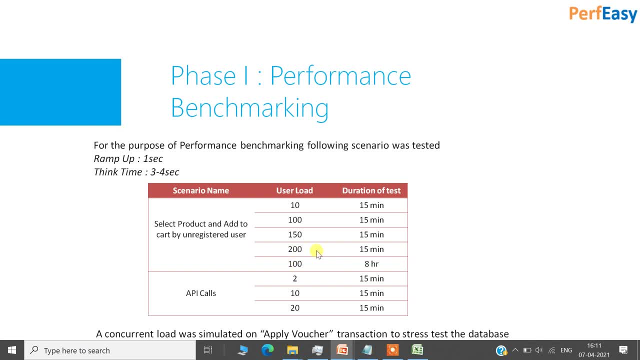 162 days for product day and we ran one endurance test for 10, 100, 150, 200, two 100 user for 15 minute test and we also ran one endurance test for hundred user for a duration of eight hours. for the api calls we ran 2 user, 10 user, 20 user, 15 minute each. 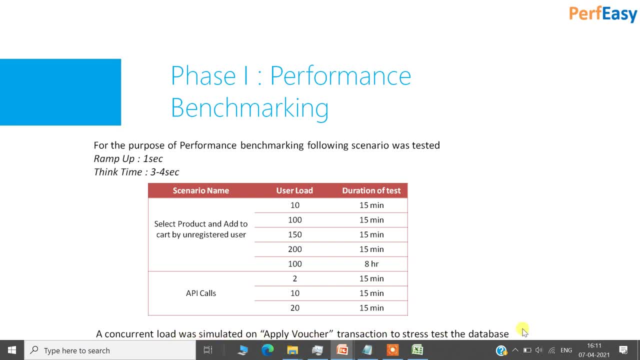 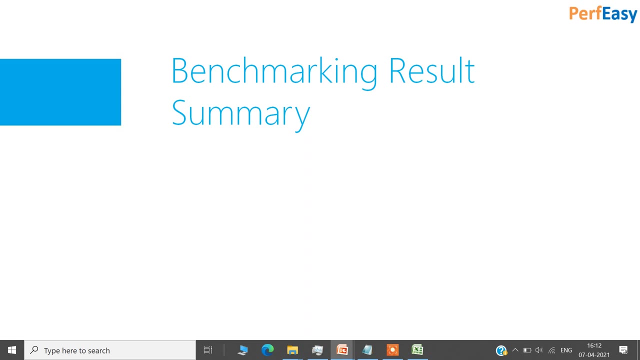 you can read the last line also, a concurrent load was simulated on apply watcher transaction to we pinpoint a particular transaction or stress test on a particular transaction to test a particular architectural component as well. so it would depend on what kind of during the user load modeling, the planning we, what kind of test we decided. now we are going to give the similar. 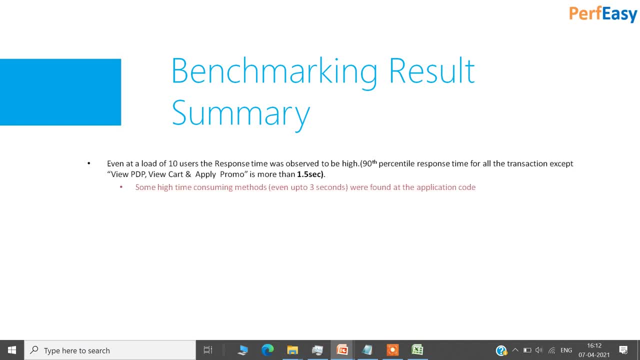 kind of benchmark result summary. here we identified that 10 users we started getting the response time more than 1.5 second. so, and during the bottleneck identification we identified some high time consuming methods, even up to 3 seconds. so at the code level application was not able to handle. 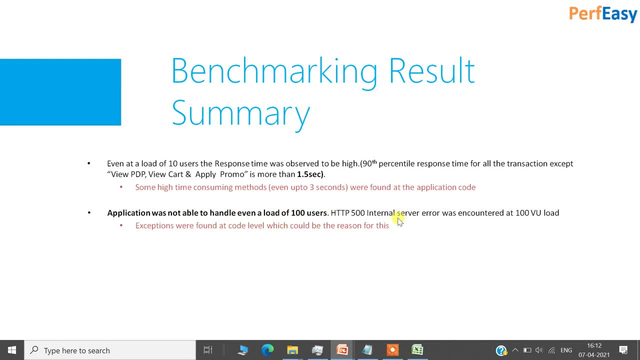 a load of 100 users, we started getting 500 internal server errors at 100 user itself. and to pinpoint or to the bottleneck identification, we identified that there are some code level exceptions which could be the reason for this. so this is a important thing that we what we observe. 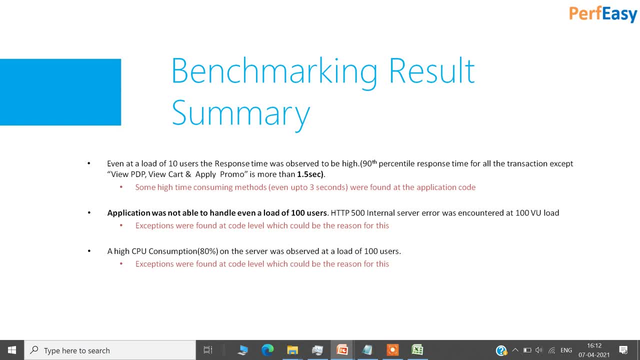 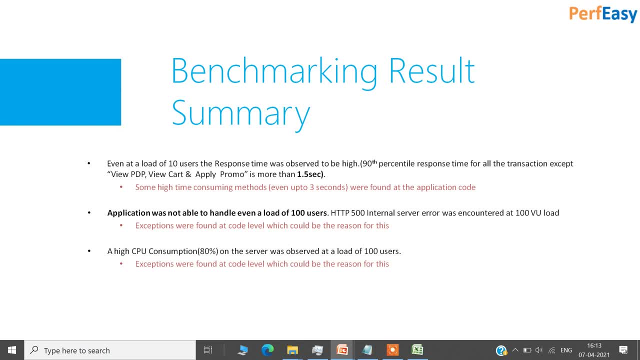 application code methods or failures, why we found out some code level issues. we also found out that the on the app server around 80% CPU consumption was happening for a 100 user load. so here some code code level discussions were found out. so because of the exceptions the logging was happening and they can be because of this the CPU can go higher. next thing that we observed was on the server side. 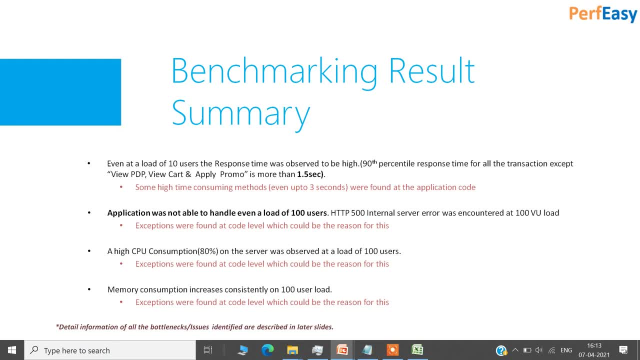 consistently. memory consumption kept on increasing during the test. because we ran for 15 minutes, the ramp-up was one second only. after one second the memory consumption the users were handed only, but the memory consumption kept on increasing. so we found out that there were some exceptions and which are the reasons for some memory issues and those things we 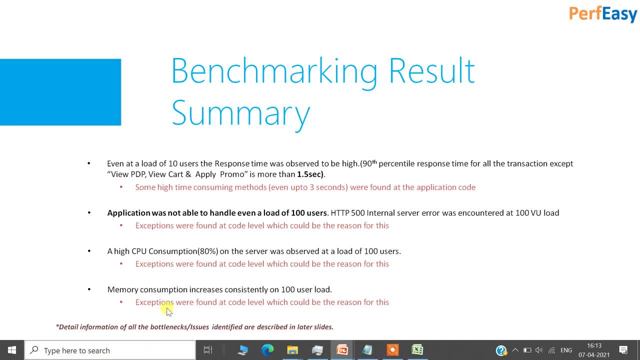 have observed in the exceptions. here we are just giving a summary and we- and the star, if you see in a detail information for all the bottleneck issues identified are described in later slide. so details we given later. here we are giving the mapping or the summary of the results. then again the same 90% response time. 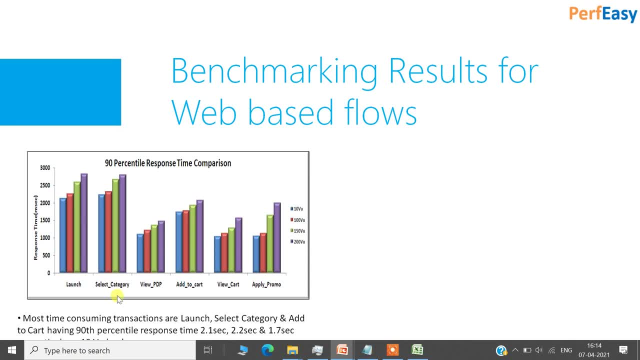 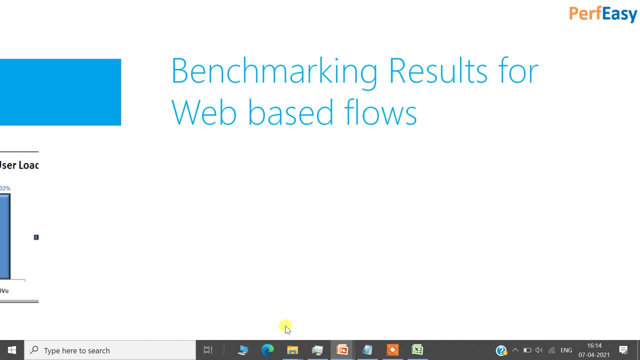 for the traction, the similar way we did and we also give- these are the transactions which are slower for two point, one second, two points over the time taking transactions. we also give the total transactions failures, the same thing that we did in the previous. so I am going to just move a little quicker. 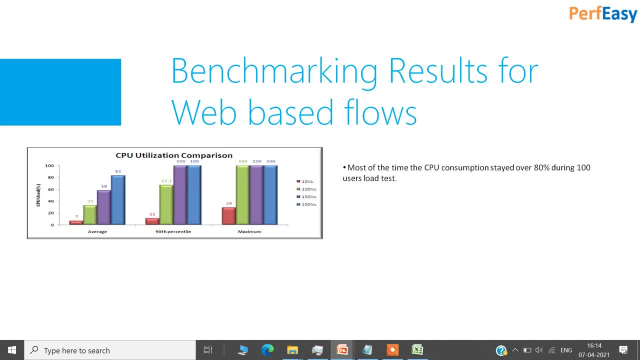 here CPU utilization, so this kind of charts we prepare that the average CPU utilization for different user load. was this 90 percentile CPU relation? is this the maximum CPU relation? was this the memory utilization statistics? how it kept on moving up slowly it kept on moving up. so if you see a consistent increase in the memory consumption, was 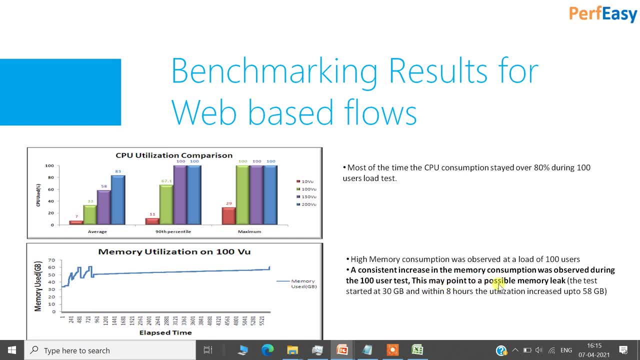 observed during that 100 user test. this may point to the possible memory leak, because the test started at 30 GB and within 8 hour the utilization goes up to 58 GB. so there was 28 GB increase in 8 hour test. this is the endurance test for. 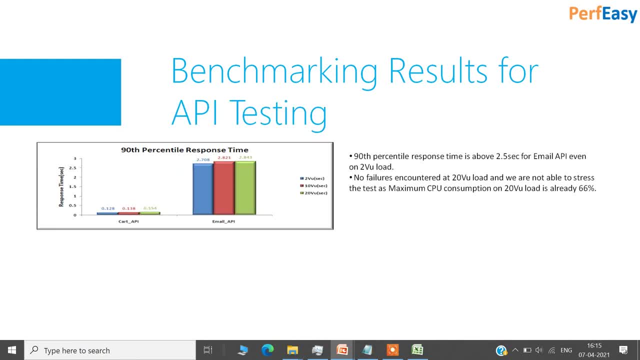 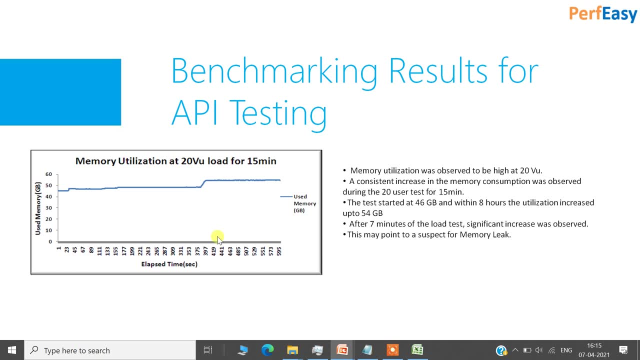 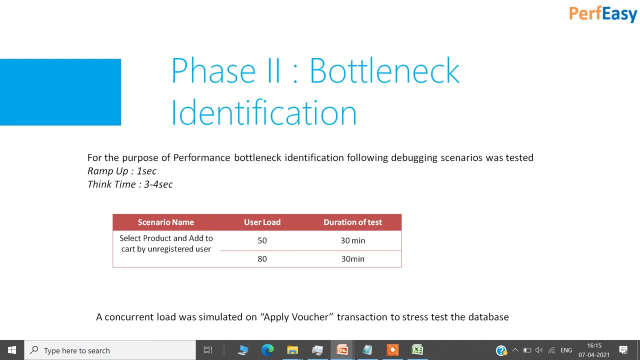 the 100 user. these are the similar data for the API results, so I am going to skip this. the memory utilization statistics: if you see for 15 minutes how it kept on increasing in the pot leg identification, the scenario that we tested was: think time was 3 to 4 second. the ramp up was 1 second. we tested for 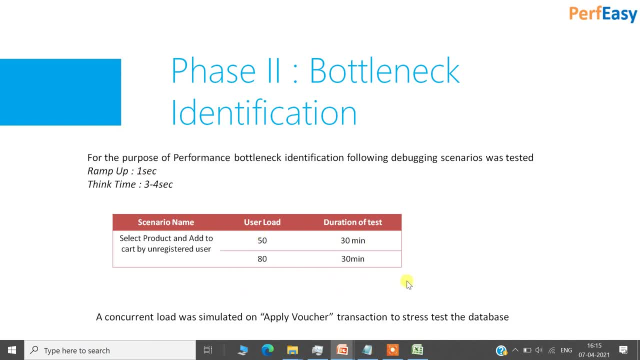 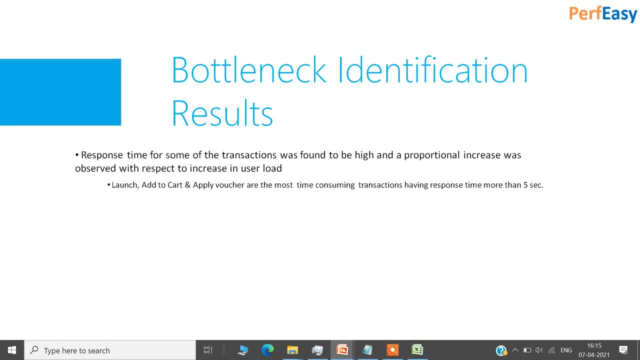 50 and 80 user. that duration of test was 30 minutes. now the result for the bottleneck identification response time were found to be high and we launch add to cart apply voucher at the most time-consuming transactions which are taking more than 5 second, some high time-consuming. so mapping this, so the time-consuming. 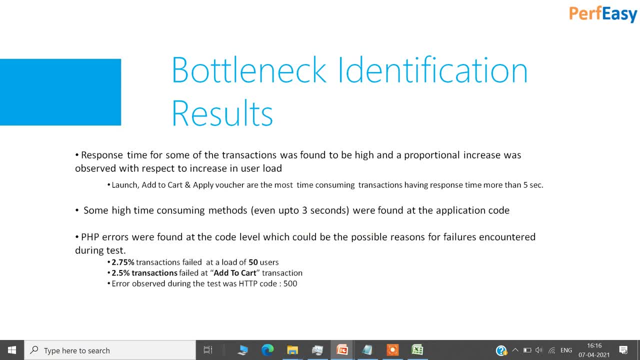 methods were found are here. we also found some PHP errors, so 2.75 percent transaction rate was high and we also found some PHP errors. so 2.75 percent transaction rate was high and we also found some PHP errors, so 2.75 percent. 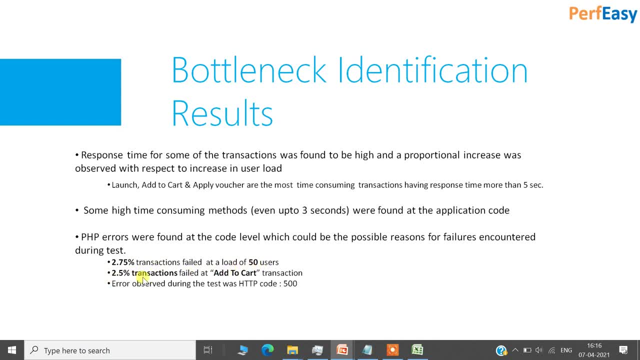 transaction failed for 50 users. 2.5 percent transaction failed for add to cart. transaction. errors were observed were 500 error HTTP code. 500 memory issues were also identified at the code level here the error messages that we found at at the back-end logs that the unable to allocate memory for full for pool was. 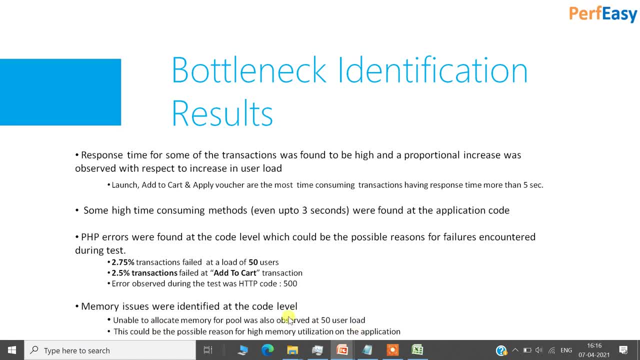 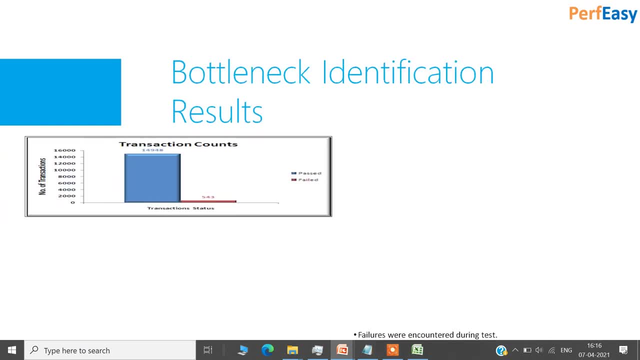 also observed at 50 user load. this could be the reason for that. the memory utilization kept on increasing. for the same balance 1 level, the transfer number of transactions appeared. the same statistics that 543 transition field out have fifteen thousand transactions and 382 stations failed for add to cart only. 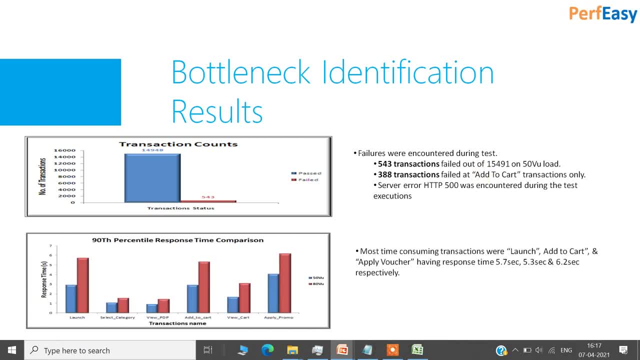 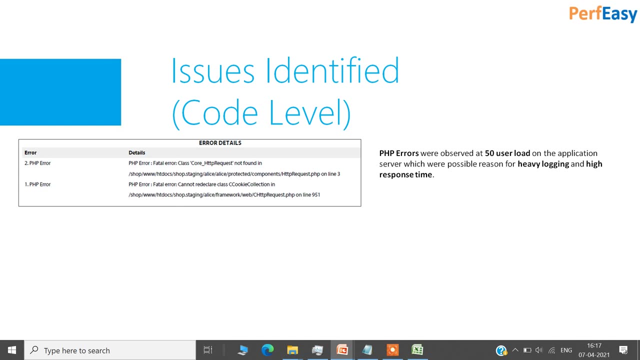 spimosum comparison by. we are giving these data of it because these tests- about identification tests were were foxed on a separate environment. so that is why we are giving the statistics again here. we are giving the errors or the issues that we identified at the code level. 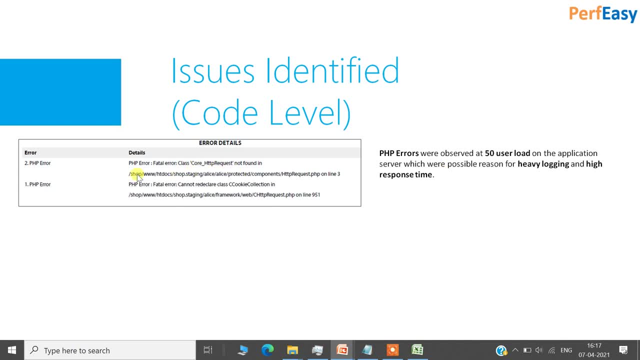 so php errors were observed. so these core underscore http request. so here if you see shop slash www http dot shop dot staging. so this is giving the complete path and the till which file: http request dot php and the line number where this exception was encountered. second, php: 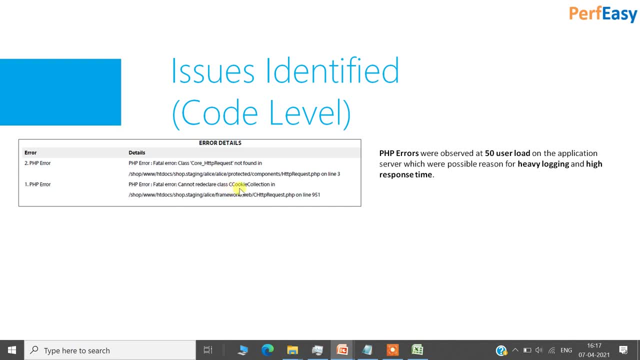 error was: cannot redeclare class c cookie collection in this file and this line number exception was. so this is where we pinpoint the exceptions. another exception where we allocate- unable to allocate memory for the pool, so this was a possible reason for the high memory utilization, and the memory leak suspect is this one. here we see the complete track trace, so that which we can. 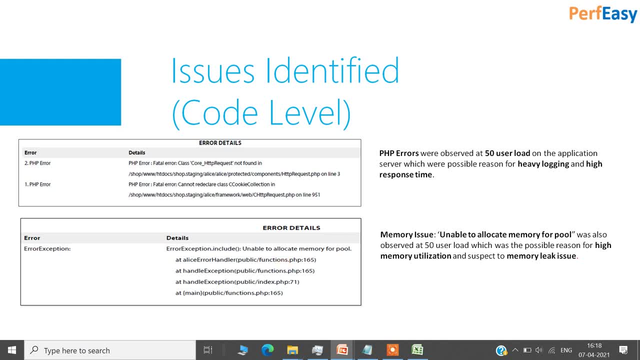 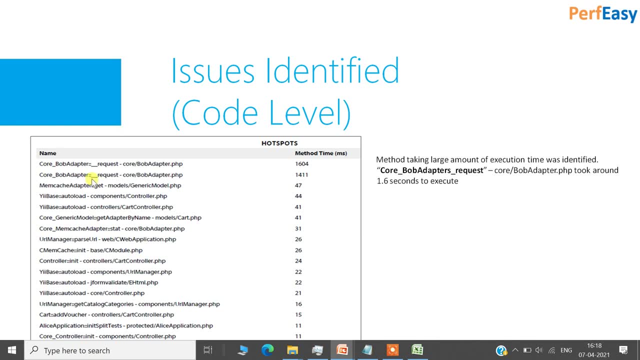 go to a particular uh uh LINE of the code and get that fixed. the code level up further issues. this is the slowest uh method if this is the core underscore bob adapters request core bob adapter dot php and it took around 1.6 second average time for the. 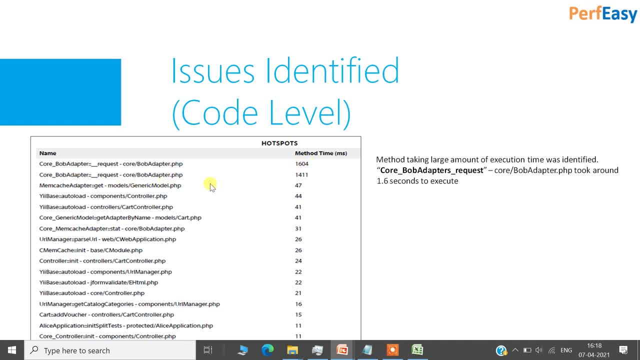 uh request. the second one is again the same: 1.4. it took up to 1.6 seconds. so here are the slowest uh method: queste, for example, memcache generic model dot php yii base is in the controllerphp so that development team can go and get those fixed. 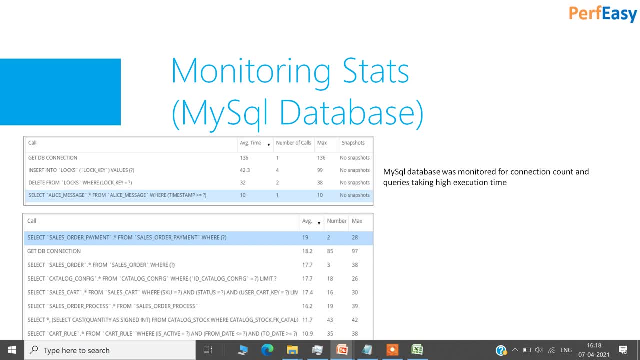 uh, the stats that we captured from the mysql database. this is the iveness rinse. this is the average time that we captured for the insert into logs queries: number of calls that were made. uh, here there were no snapshots. these are the database queries that are taking time below. uh, the queries that are are also the queries that are showing up in this video. 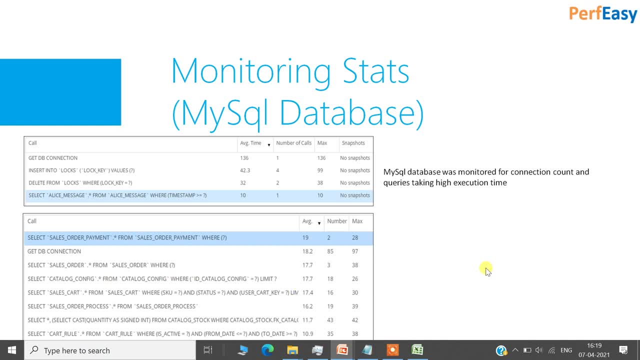 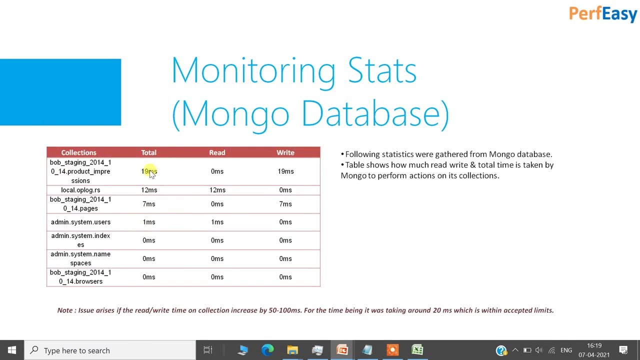 uh, uh, end, uh, end, end, uh, that are taking time. This was note down. please note down. this was the MySQL database statistics and now we are. we also shared the MongoDB statistics: The number of reads that happened. sorry, the total that happened for the connection wise, the number of reads. 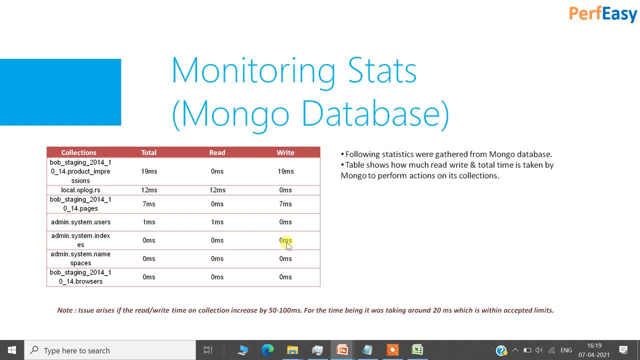 time that took in millisecond the number of the time that it took. Issue arises if the read-write time on collection increases by 50 to 100 milliseconds. Here we should also give some reference values: This: 19 millisecond, 12 millisecond. these numbers are not giving. 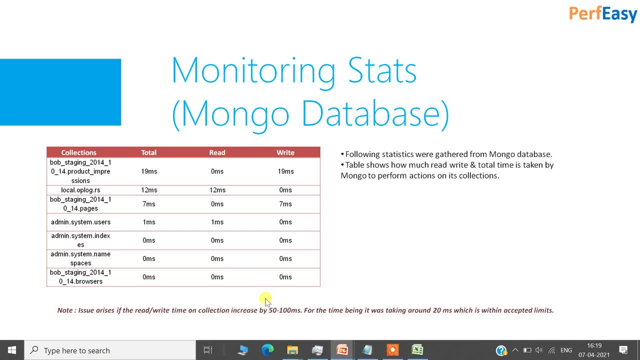 any reference value. So here we are also giving the reference value. If it is goes around 50 to 100, then it means that it is problem. But here we observed up to 20 milliseconds, so that is under acceptable limit. So there is no issue on the MongoDB side. 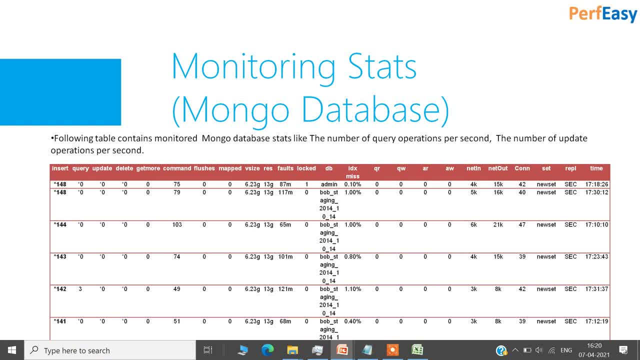 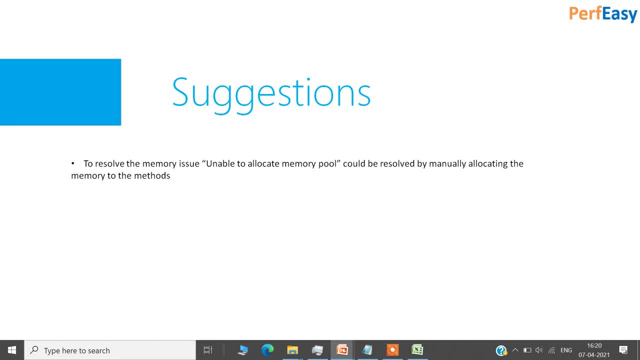 Some more statistics that we captured on the MongoDB sites And in bottleneck identification activity. the another important aspect is to give the suggestions for improvement or the fixes. So here we should. we give them session like resolve memory issue: manually allocating the memory to the methods so that methods 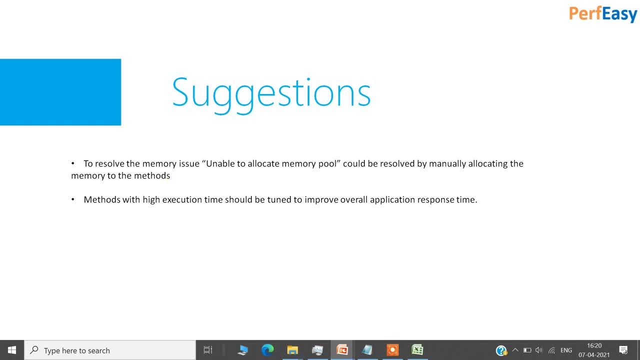 have more memory available so that this unable to allocate memory issue is not encountered. okay, method with a high execution time. we have given the to pinpoint till the code level and the line level of on the code so that those methods should be fixed. we. 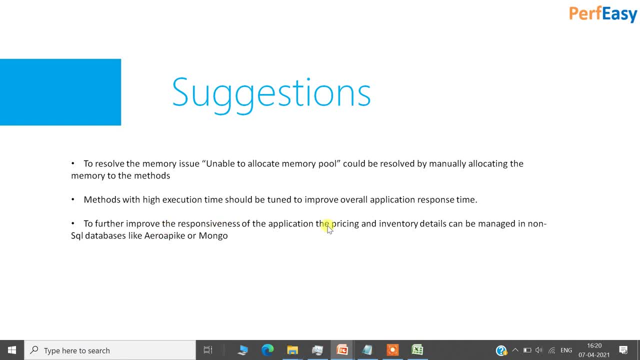 also suggested that, to further improve the responsiveness of the application, pricing and inventory details can be managed in non sequel database like arrow spike or MongoDB. for logged in user, the card detail should be saved in MongoDB so that the time for my sequel loading takes is ignored and as the 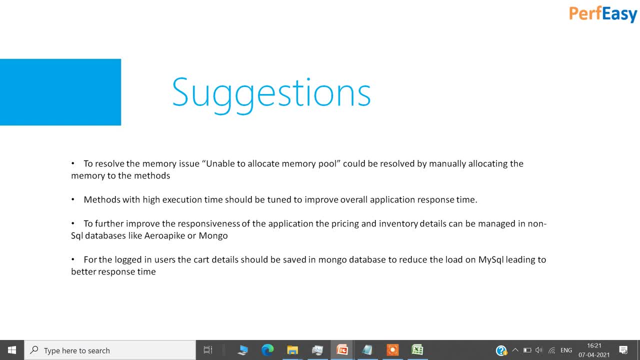 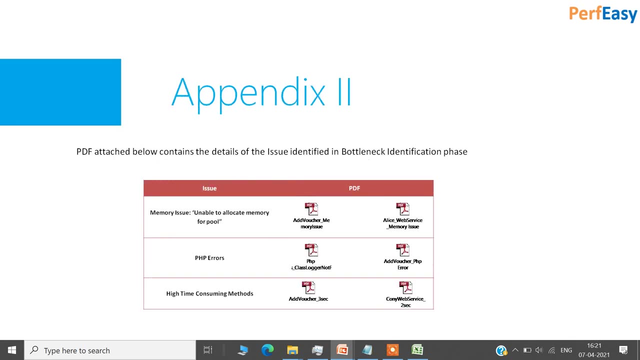 MongoDB is comparatively faster and which would lead to the faster response time in the cart information, and we can also reduce the load on the my sequel database. so by moving the fishless data into the MongoDB. so we also shared the complete stack trace of the memory. issues a PHP error, the high-consuming method with the 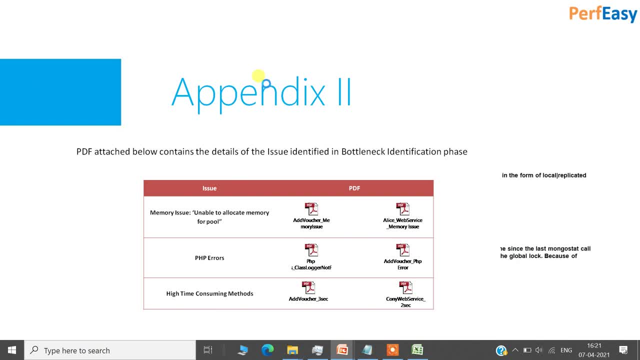 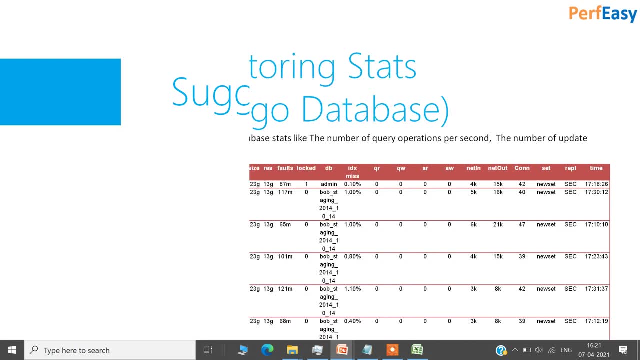 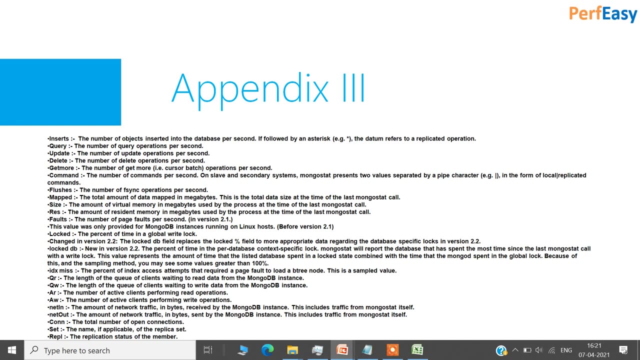 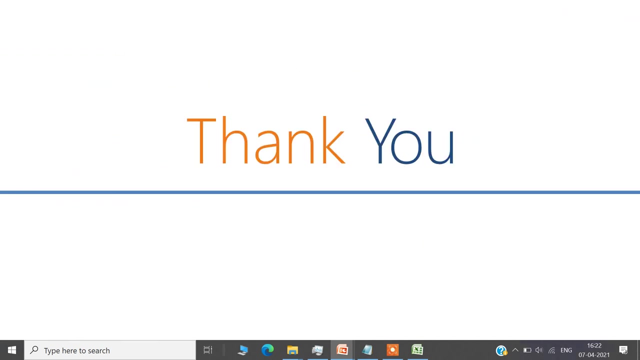 development team, which we presented as appendix. so these are the relevant data from the. I showed you know this table, so what is this query? update, delete. so these are the. in the appendix 3, we have given those reference data so that people can see what is the meaning of those values. this is the bottleneck. 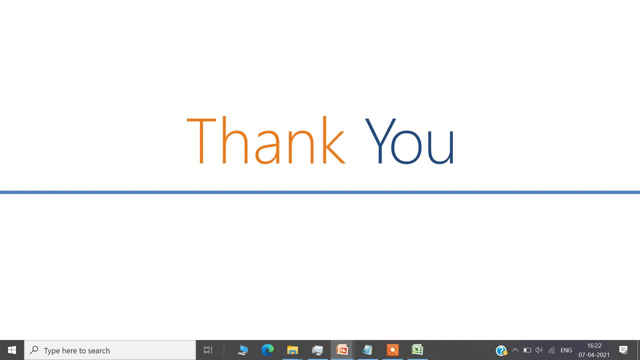 identification report hope you have. you have you will get benefited from these reports, the type of reporting that I presented. I would like you guys to also share your experience. if you think that there is any other statistics from the benchmark or the bottleneck inclusion report that we should also share, please. 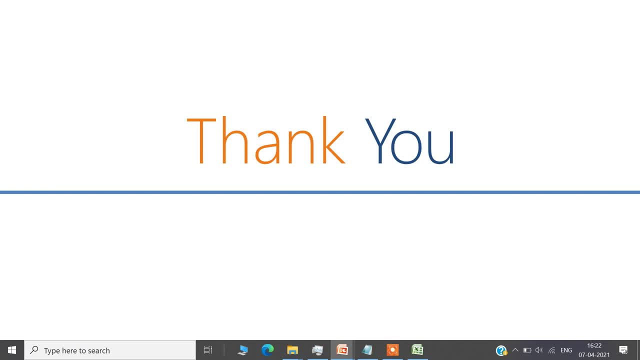 mention in the comments, so that other people also get benefited, because knowledge increases when we share our data and we share this information. we are the knowledge.